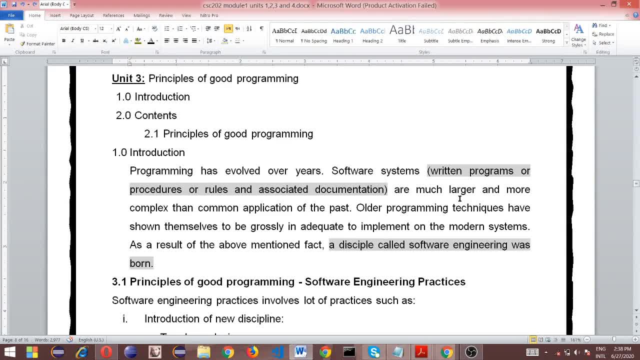 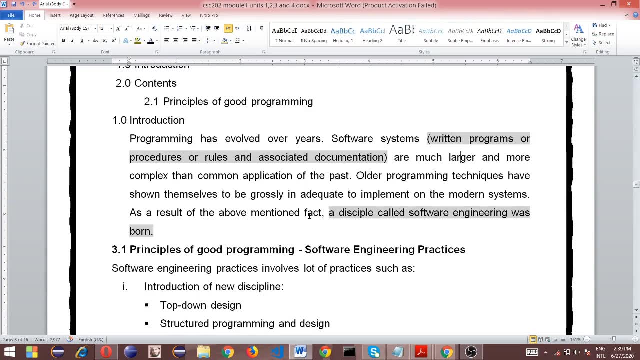 Then common application in the past, for example. So there is a need for us to have a kind of principle. So this resolved into what we call the software engineering principles of good programming. The idea here is that actually programming started with a very few codes for a software. 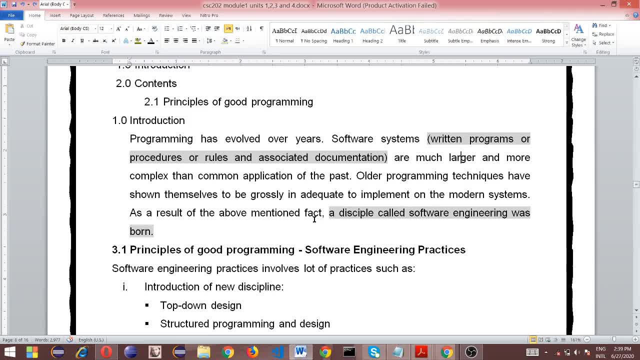 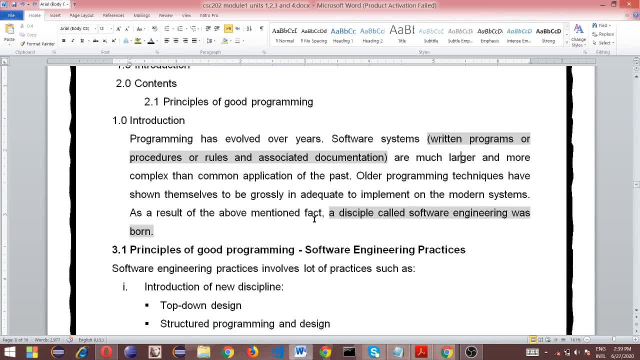 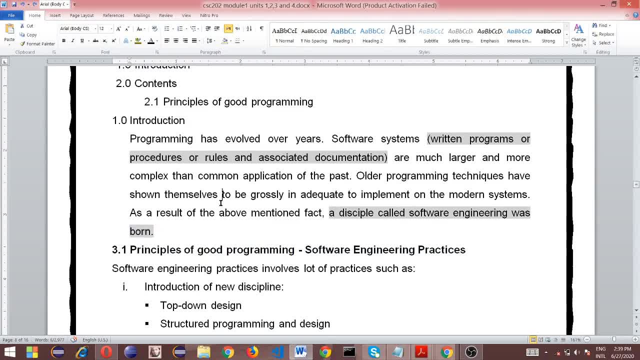 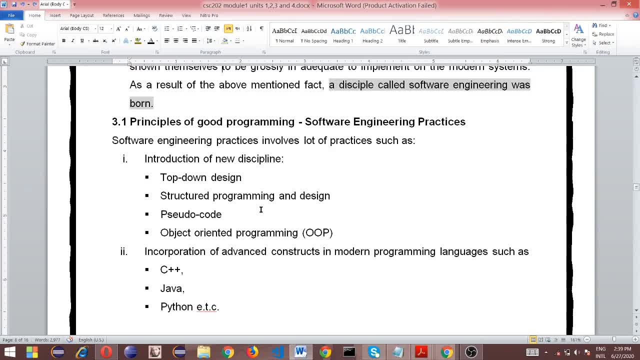 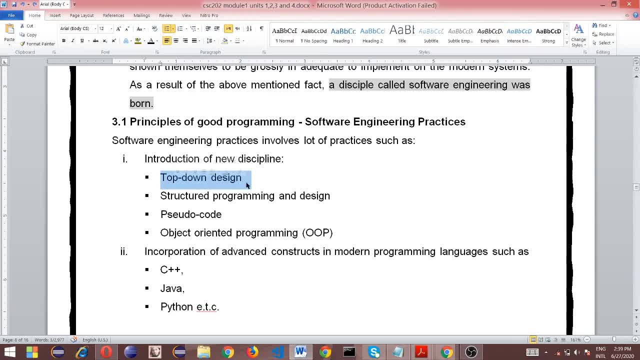 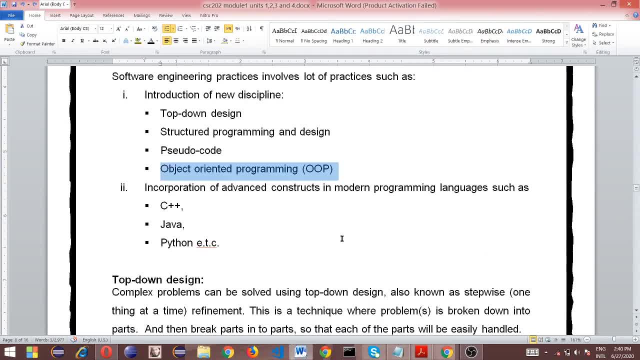 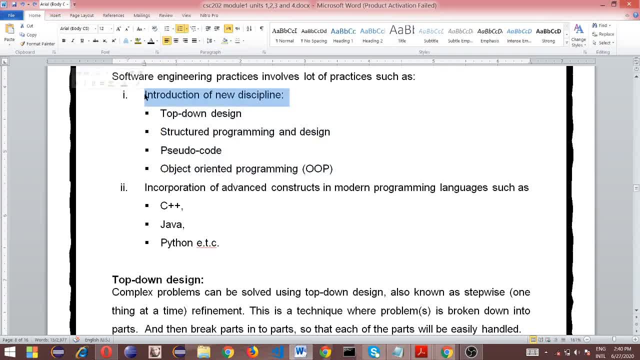 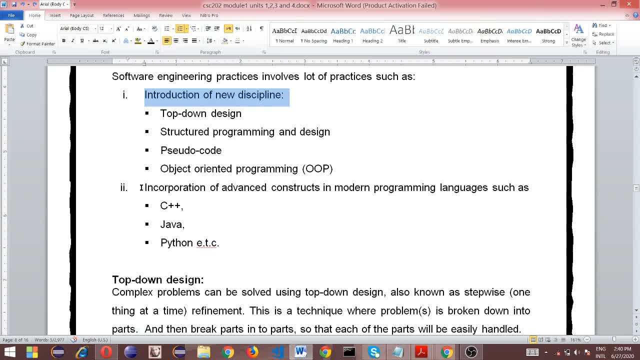 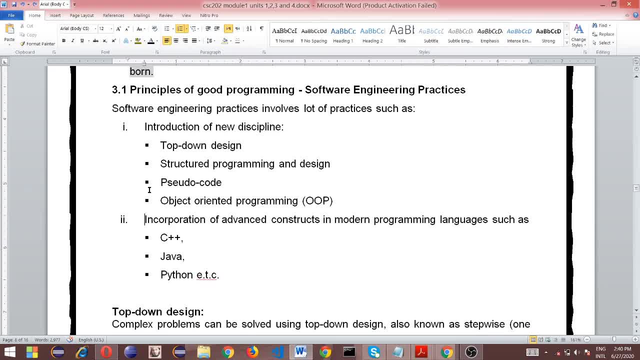 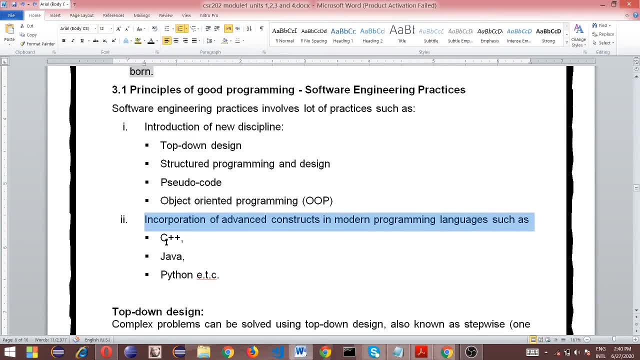 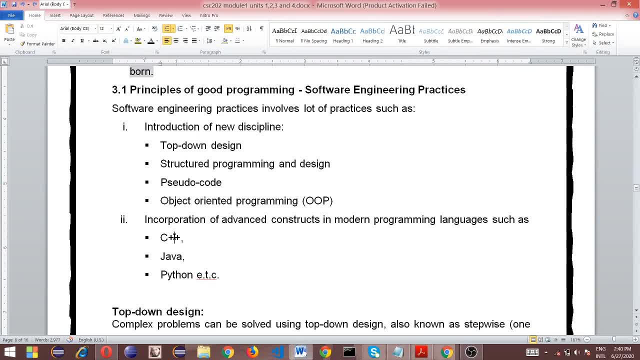 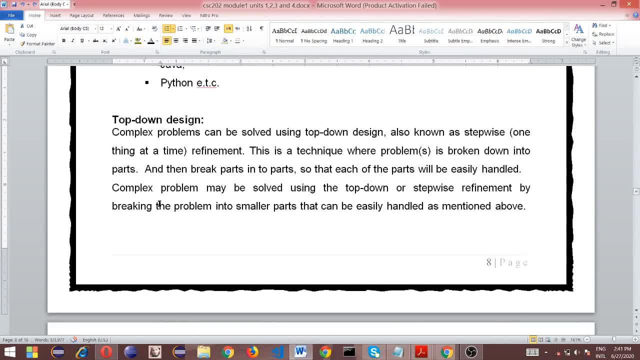 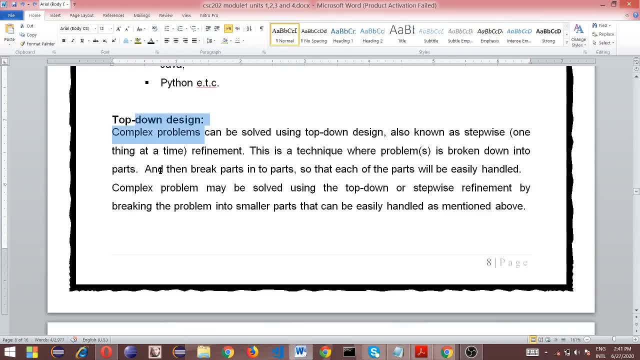 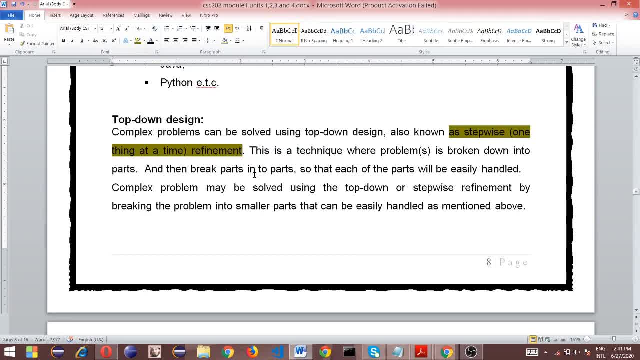 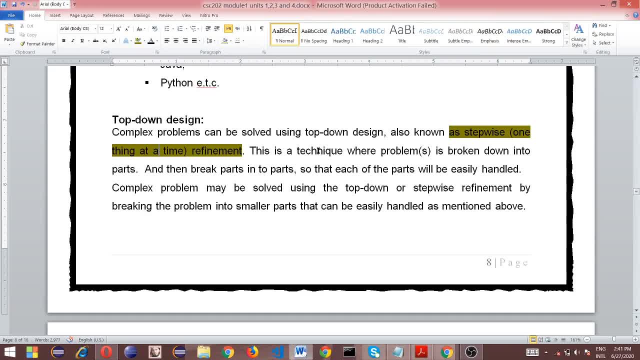 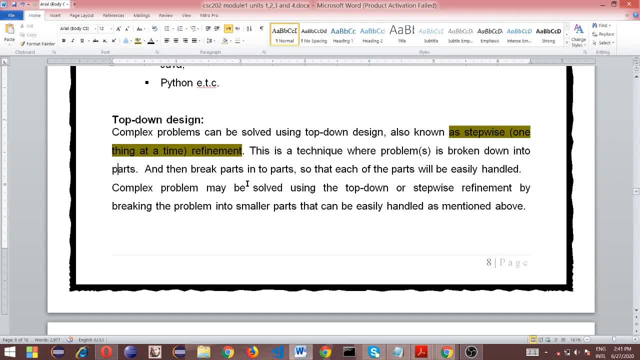 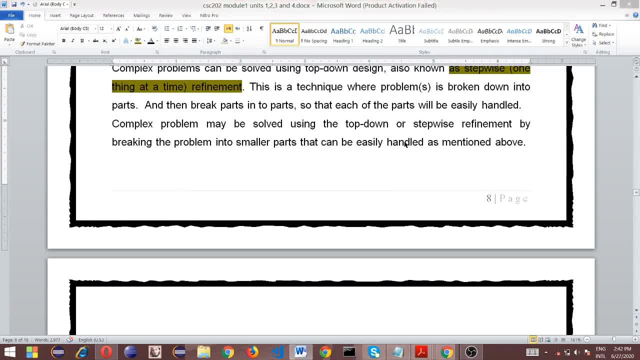 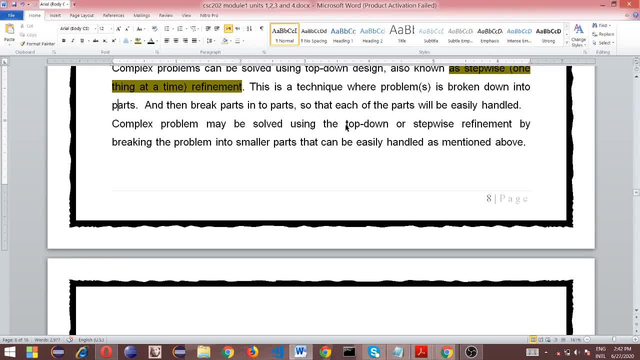 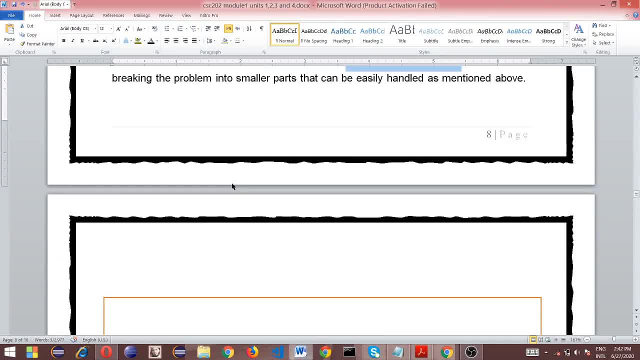 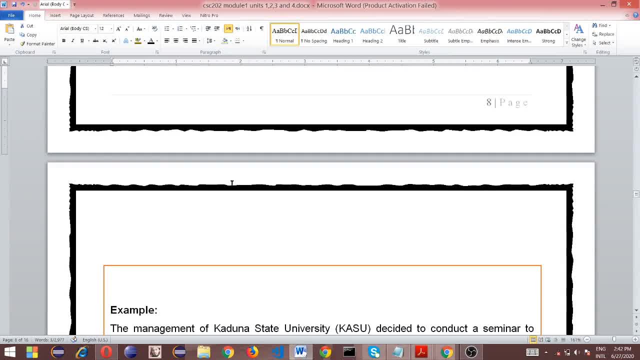 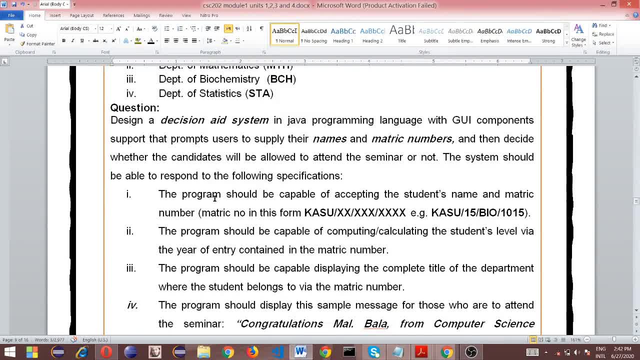 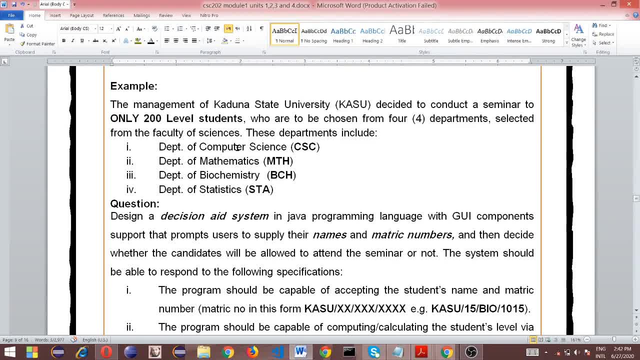 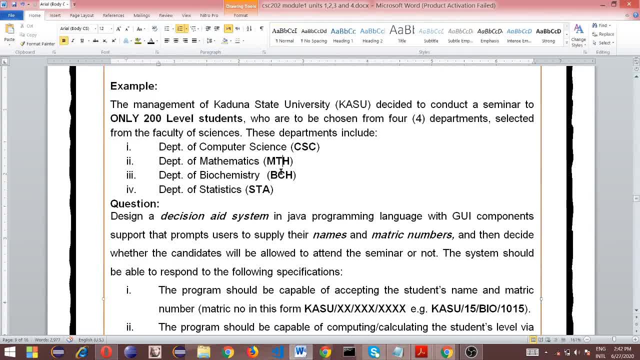 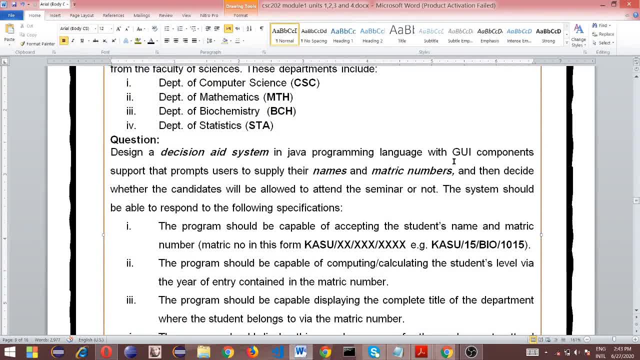 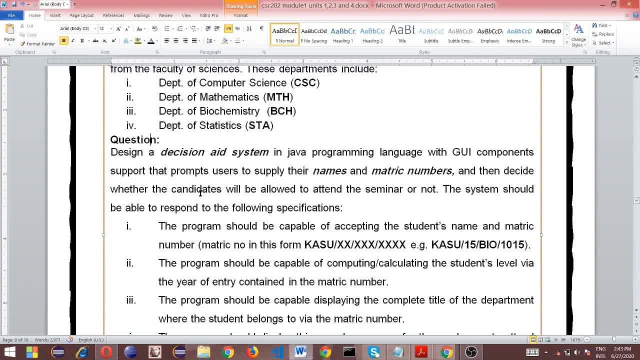 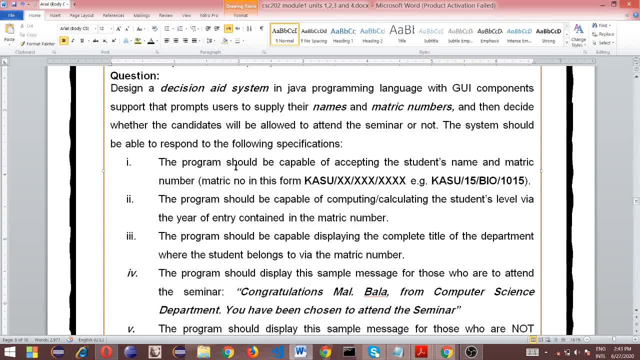 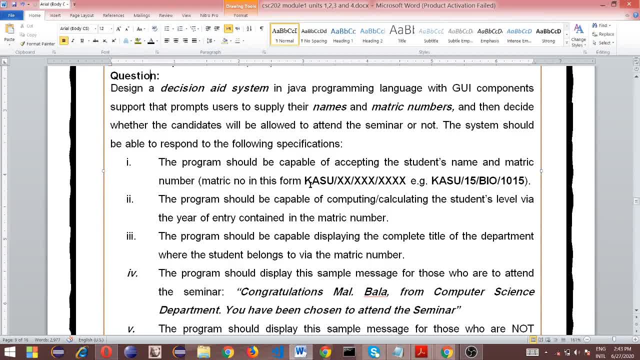 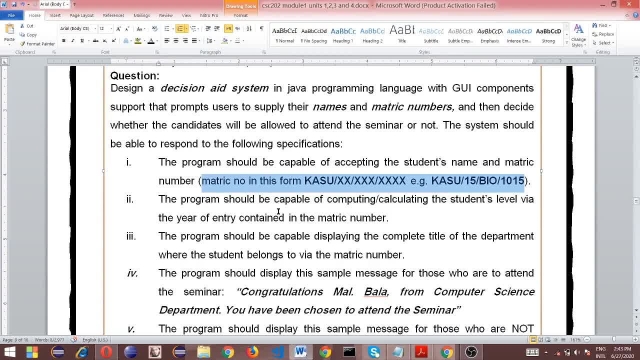 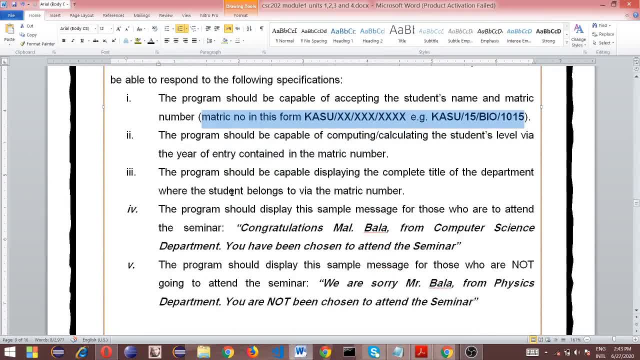 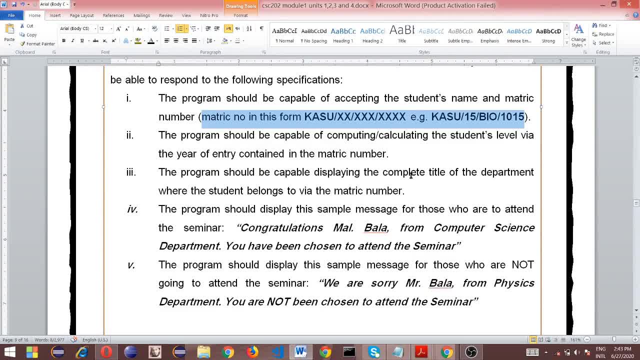 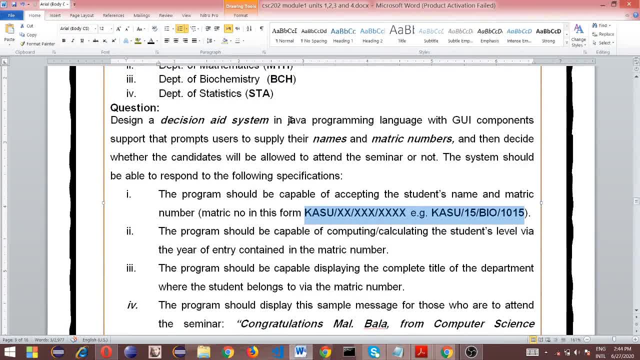 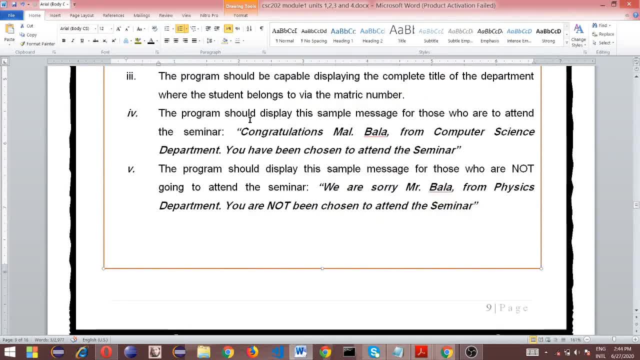 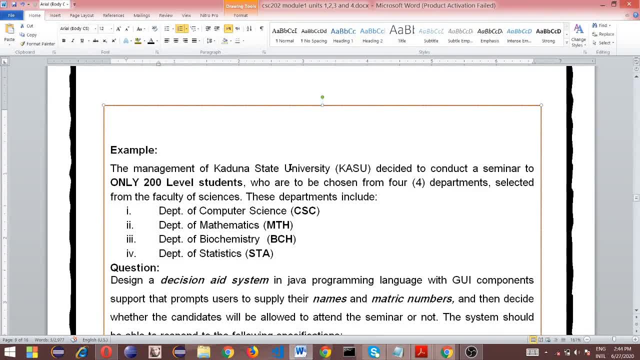 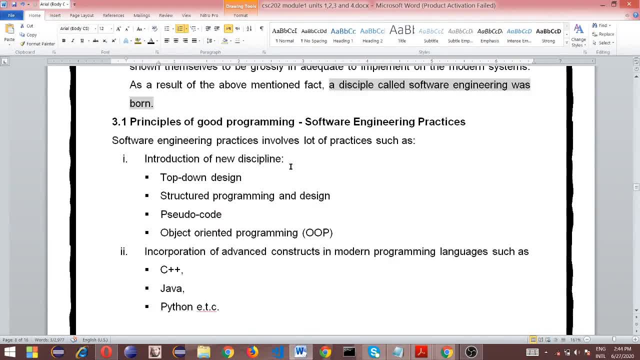 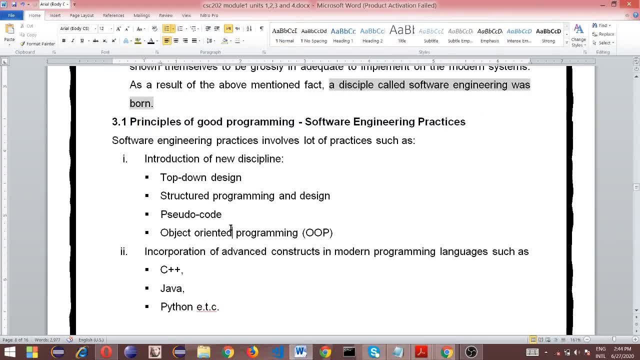 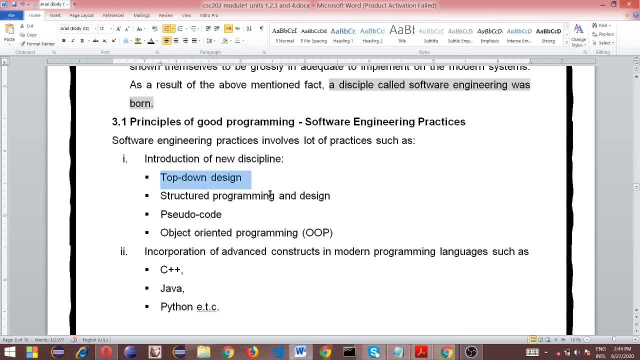 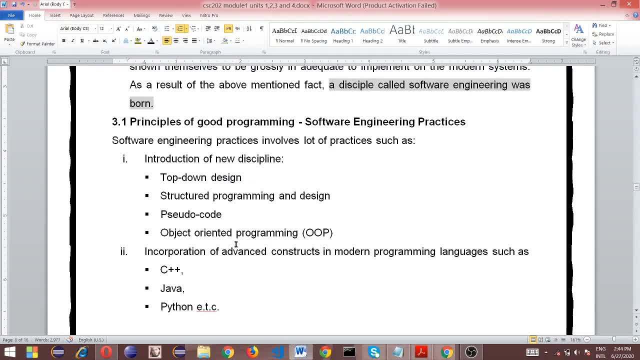 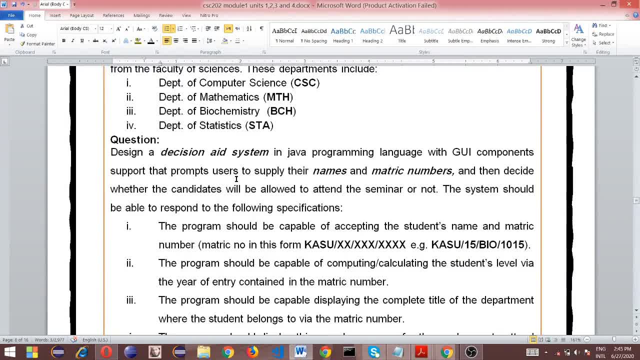 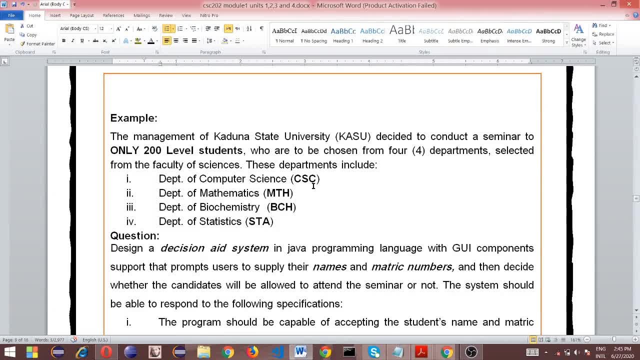 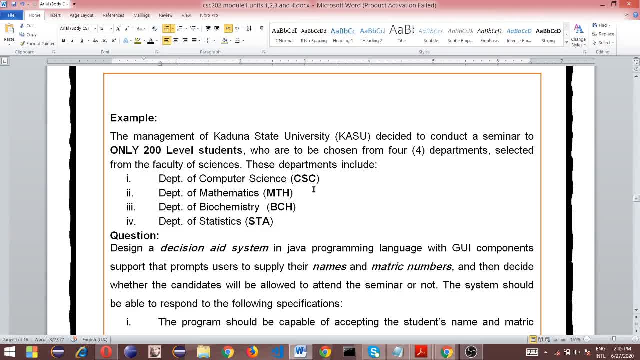 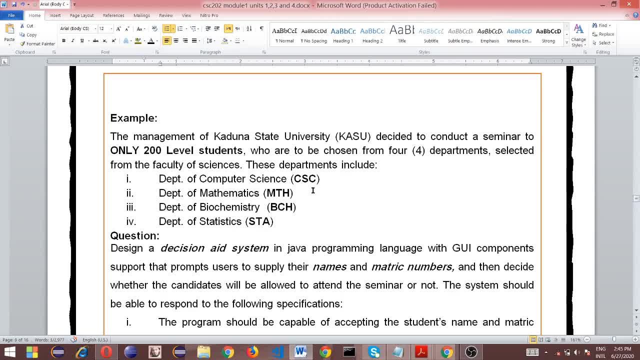 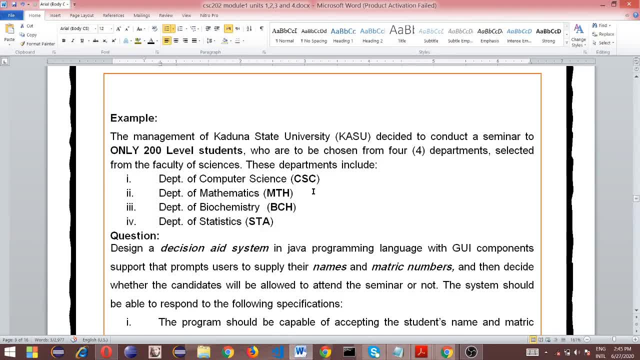 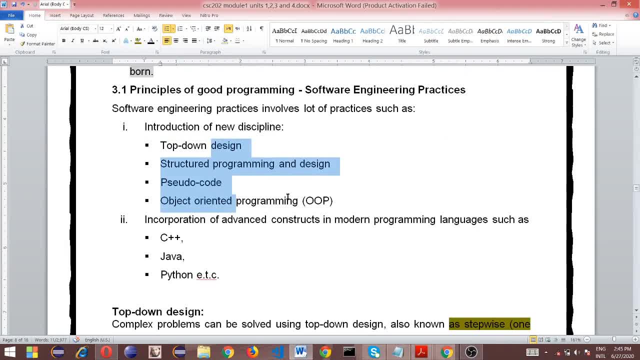 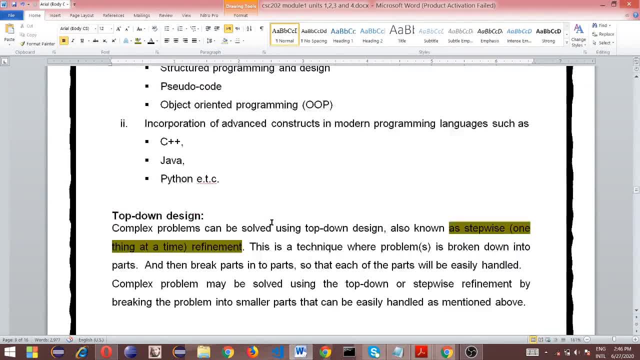 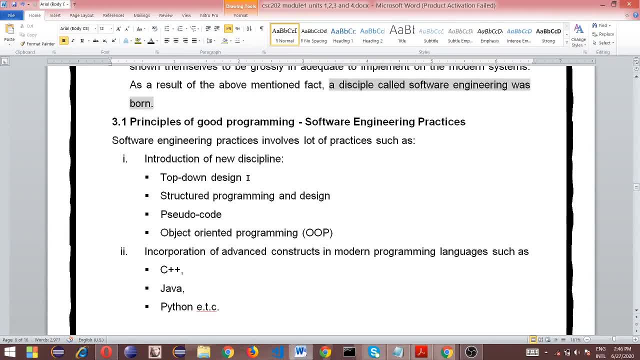 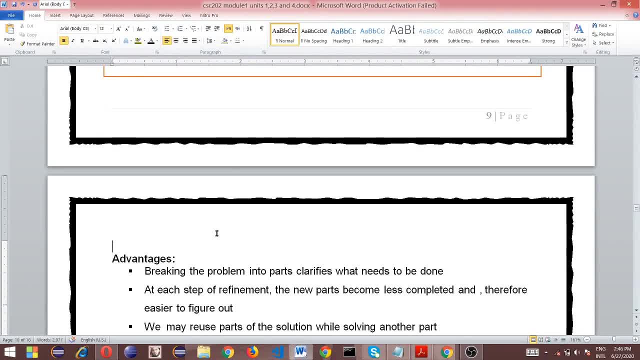 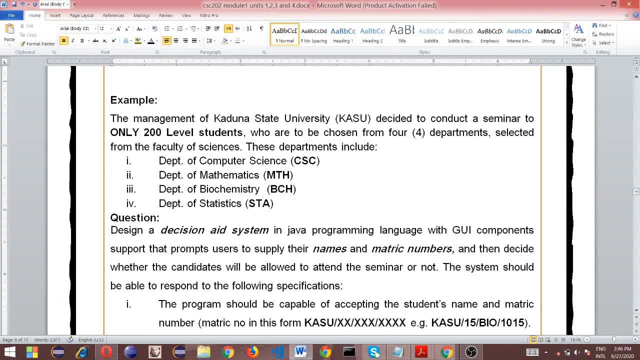 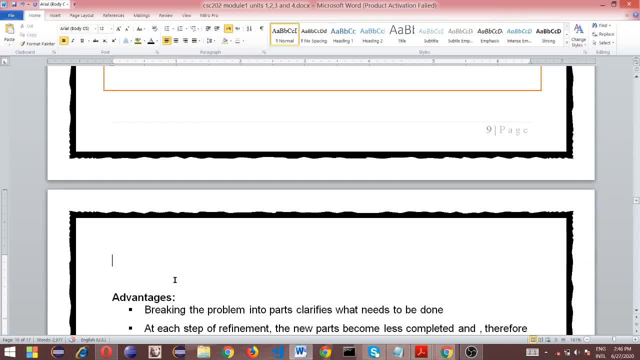 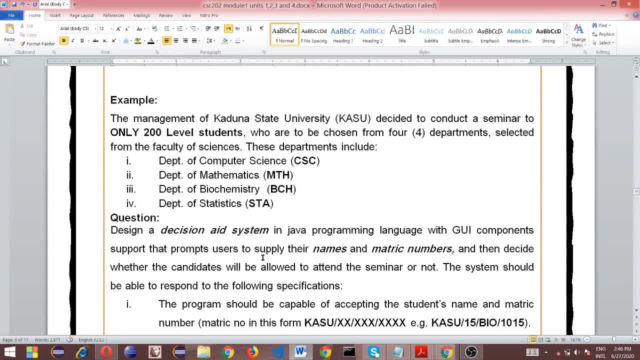 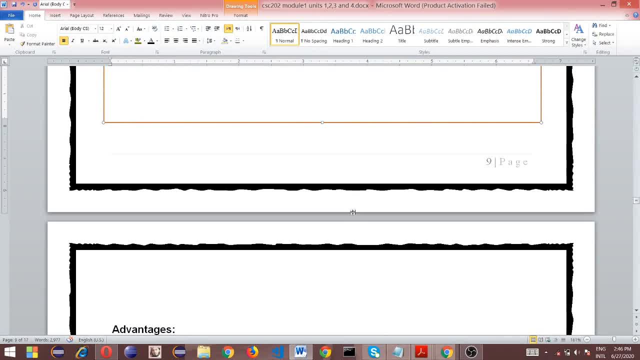 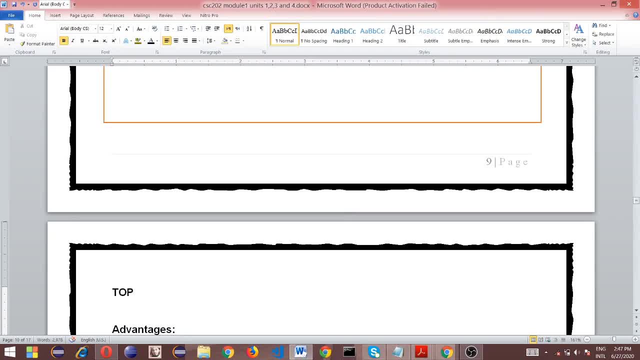 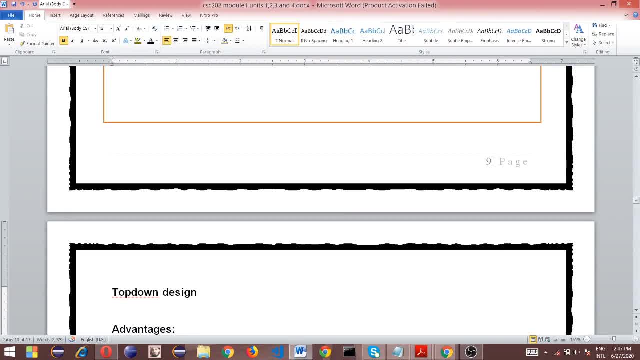 So you go by if you go by top down design, For example, and then you've chosen base. 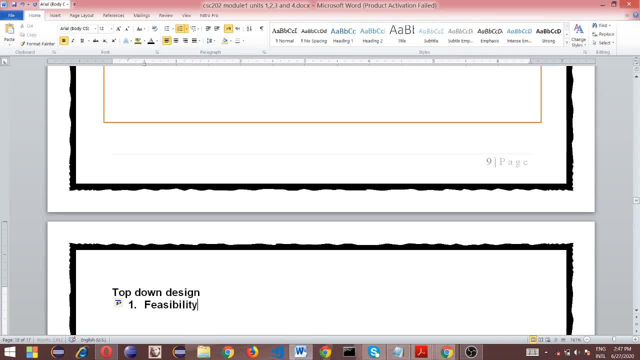 But first of all, you do visibility. Visibility studies. This is based on software engineering Visibility studies. You study the problem, try to study the problem, and you have to have a conclusion for you to Continue from. 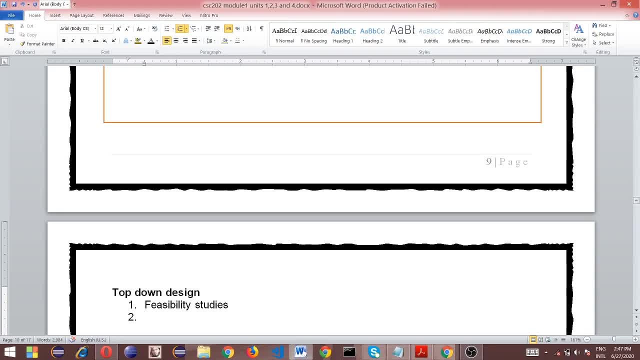 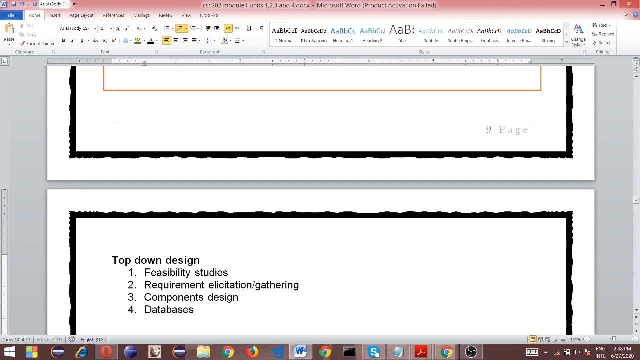 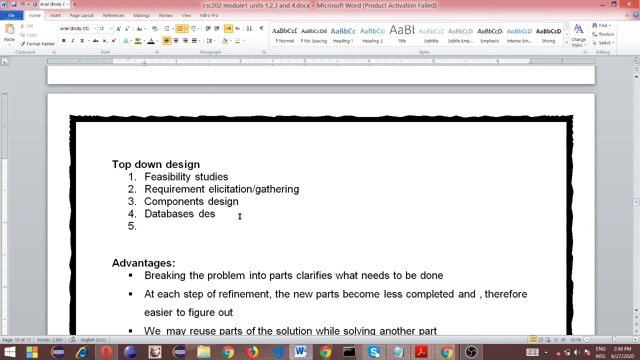 disability studies there has to be a conclusion conclusion that computer could be applied to solve the problem or computer programming could be used to solve the problem at hand and from there you go by requirement elicitation what are the requirements for the actualization of the projects so you have to elicitate or requirement elicitation or gathering you gather requirements for the program and then you go about the component design then you go by the database design then you go by the unit integrations component testing design then you pick units 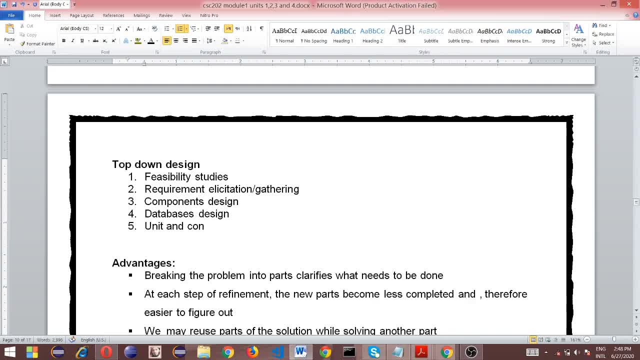 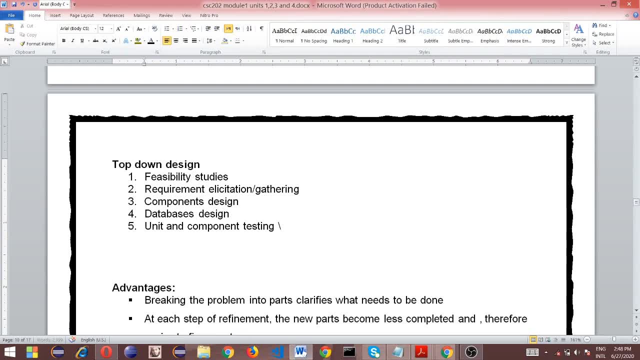 and component component testing then you pick your component integrations when you test all components and they're they're okay working correctly then you implement unit and component testing 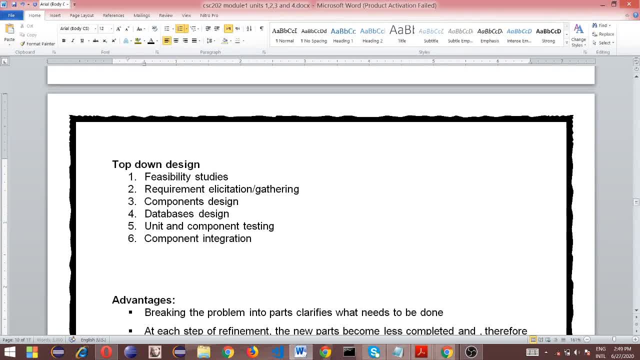 then you integrate the component and then uh 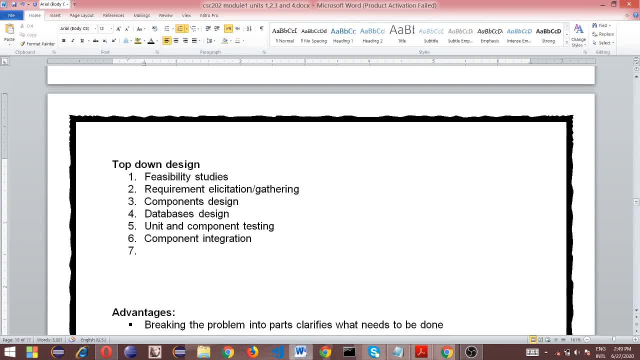 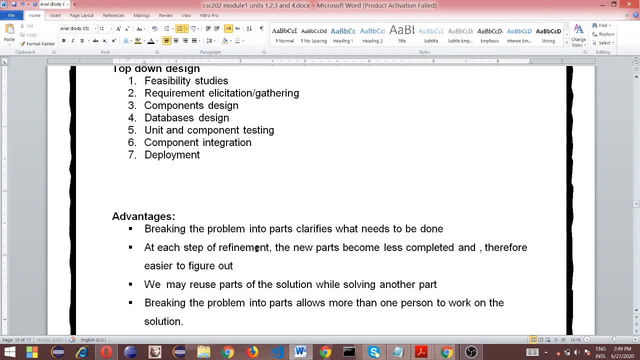 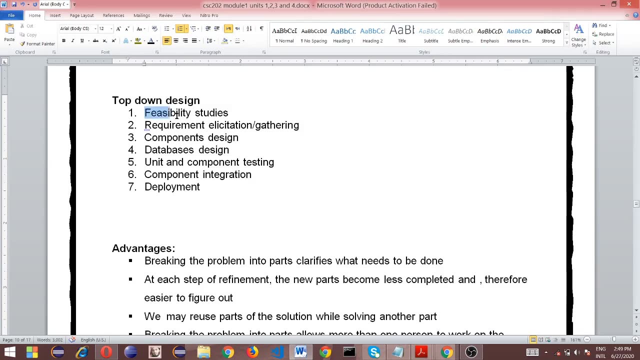 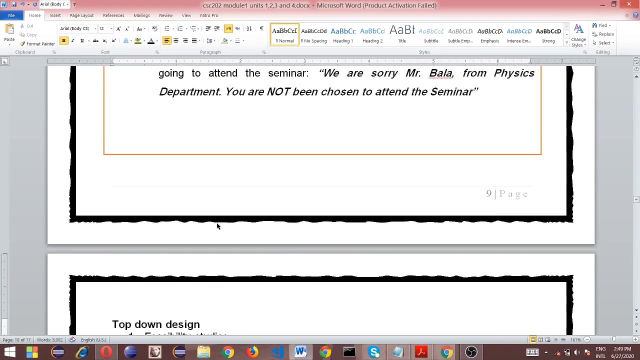 software deployment and all that so this you've broken down the problem into sub parts and each and every part could be handled by some kind of some professional this is what we call on the top-down design you can also use the concept of 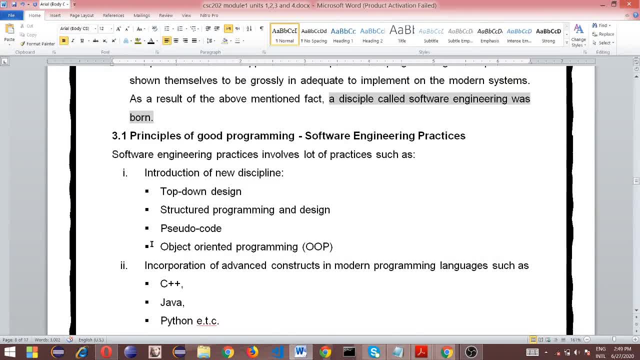 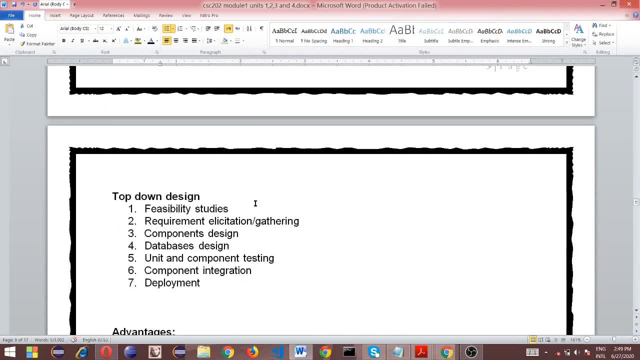 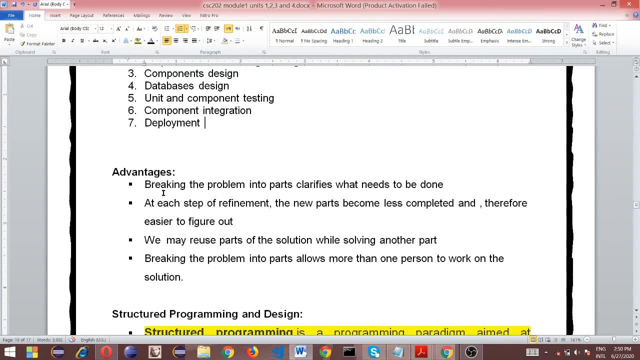 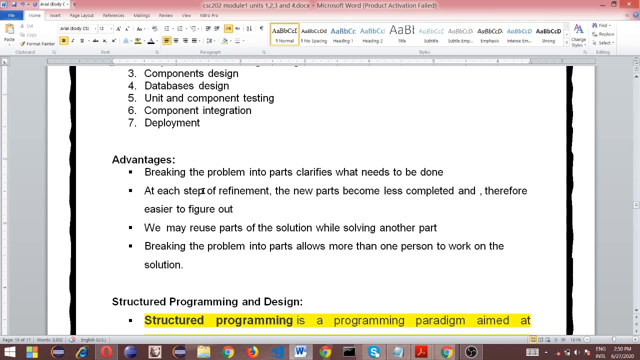 OOP to solve the problem by using objects now you represent all these but with some kind of objects and then you introduce the OOP principles and you begin to call and and work with it actually this is somehow high higher than your level but then you need to know this so advantages if you have these 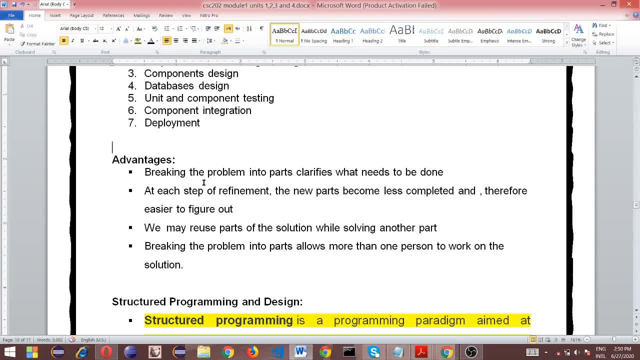 principles of good software practices good software practices you have these advantages you broke the problem into parts it clarifies what you need to be done at each step you refine and then path becomes less complete complete and therefore easier to figure out and then we may reuse parts of the solution you can reuse part of the solutions the solutions to problem number one and the solution to problem in a particular stage could be used when needed and then you could also break past the problem and then this allows more than one person to work on on a project or on a solution and that brings about integrity and more reliable future all right 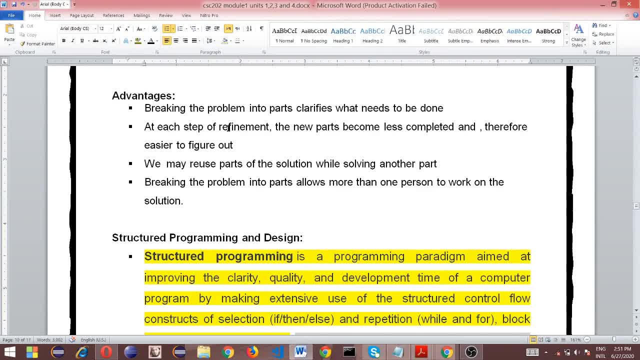 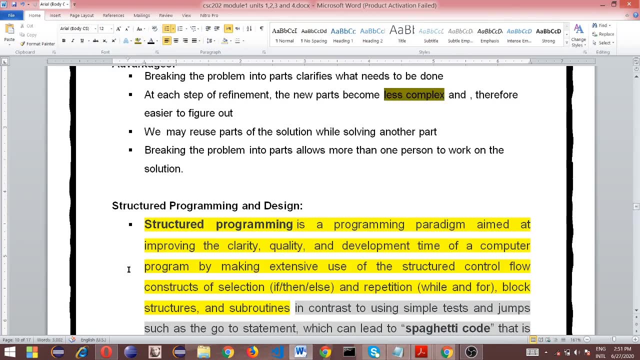 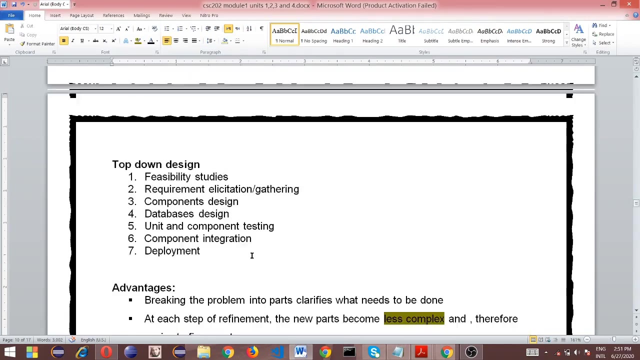 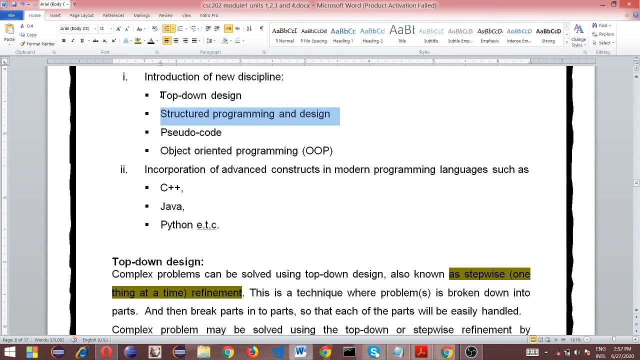 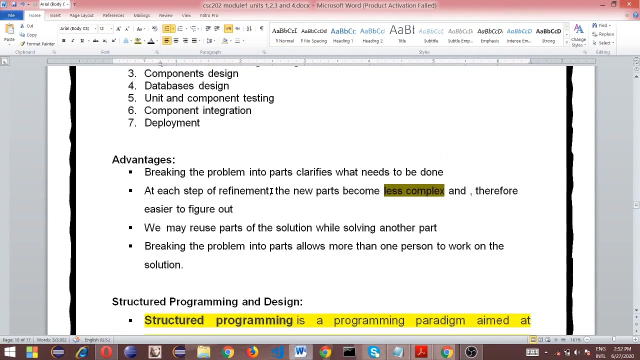 actually there is a mistake here at each step of refinement the new parts become less complex it's not completed less complex I'm sorry another mistake here less complex structured programming design you know we mentioned some kind of disciplines that could be used here structured programming design I'm going with top-down design so now you can use structure structured programming design as part of software engineering 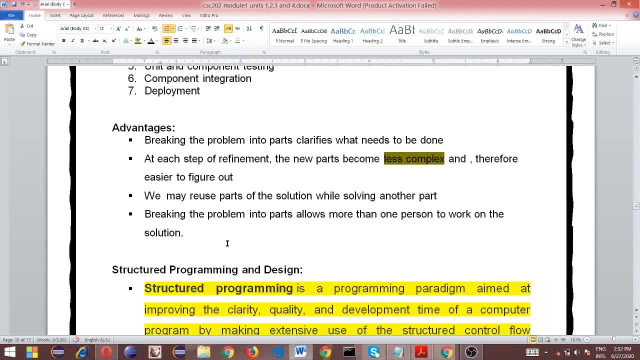 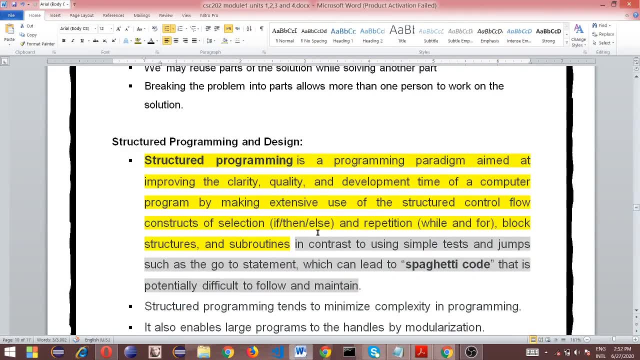 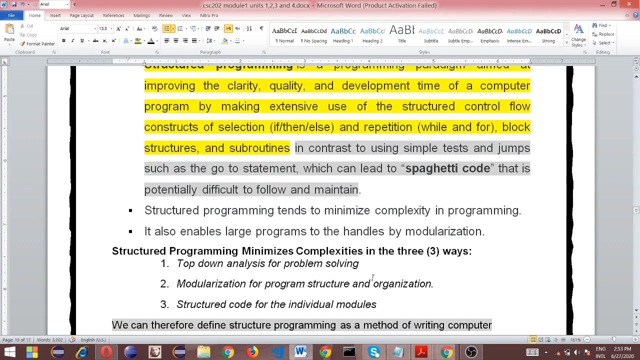 good practices you cannot just start solving problem without picking a particular pattern so structured programming design you need to know what is programming structured programming for the first time actually structured programming it's one of the programming paradigm that aims at improving the clarity quality and development time of a particular computer programming by making extensive use of structured program or structured flow of programming and when you talk about structural flow of programming you're talking about the selection we're going to discuss this later just in this video talking about the selection the repetition and that's the Quence and then it it also talked about the root and and all that so structured programming tends to keep programming a very good shape and good structure such that things like spaghetti coat or not will not be seen in the program please trying to find out about this because if you use structured programming sometimes the bloopers use a statement code go to statement and this go to statement next programming to look like 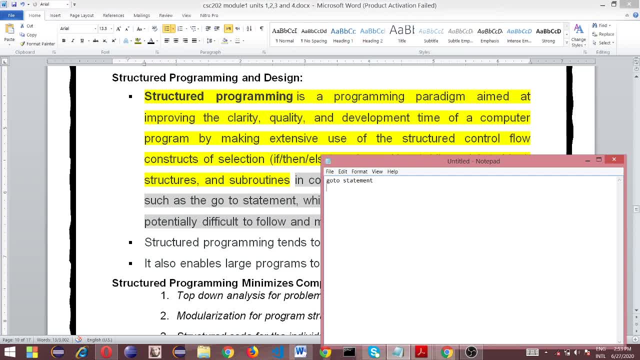 this pateko you are ascending you know when you construct a particular when you struck the execution of the program from one line of code to another line of course on a line of course imagine if you are working in a team mr a instructs a program from line number one to line number 10 while 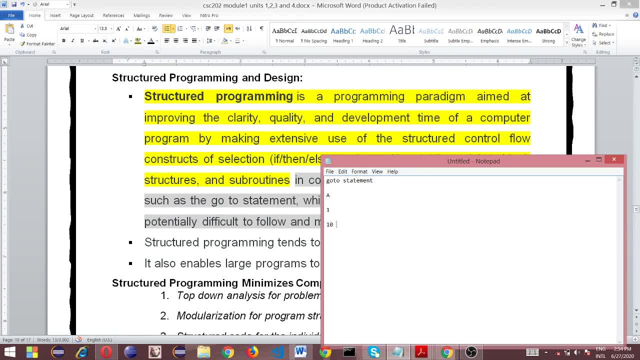 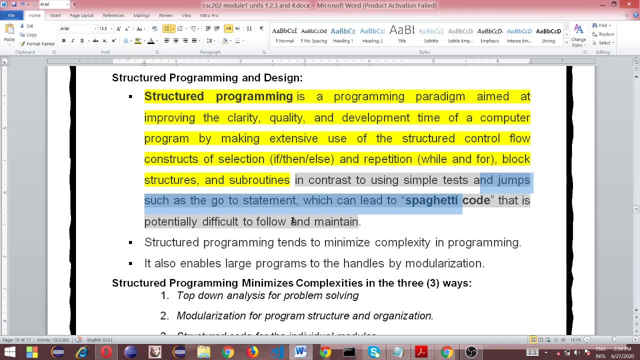 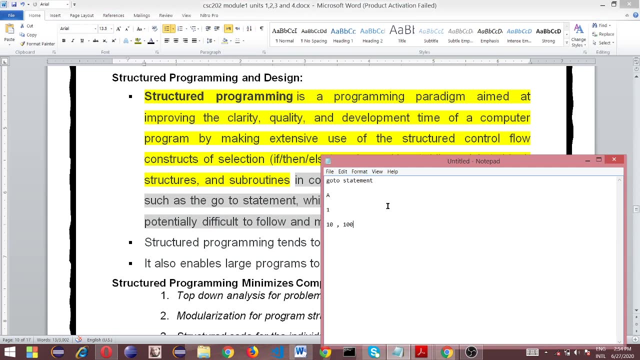 mr b for example at line number 10 instructs the program to line number 100 what will happen there could be issues so this is a kind of programming in which structured control 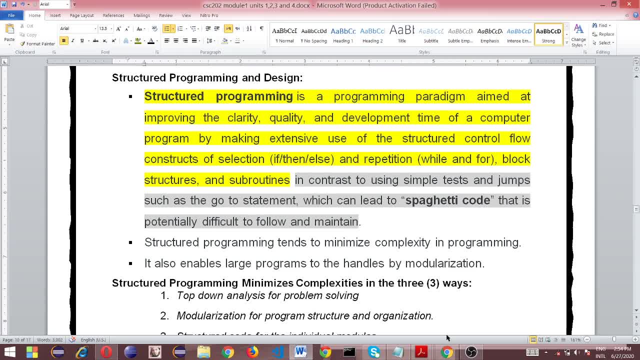 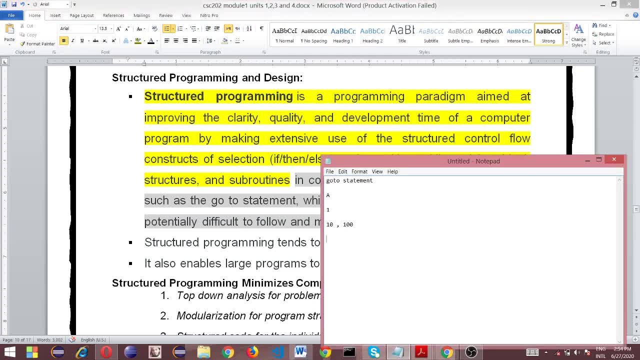 structures are not in place that's the reason why the jacobini and on the somebody bohong we shall see in this presentation came up with the introduction of a theory of structured programming 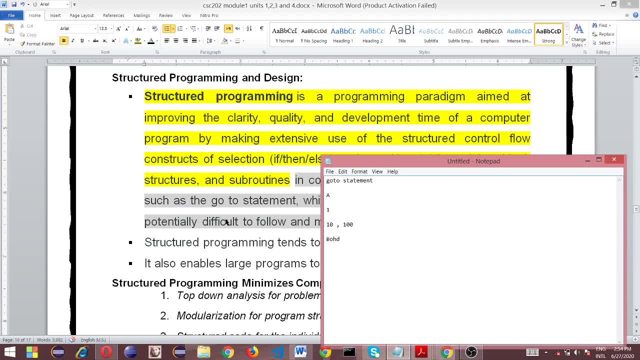 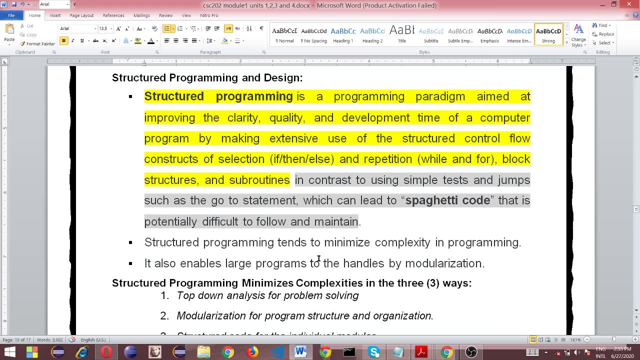 and they abandoned developers were asked to abandon the former way of development so they had to imbibe the new 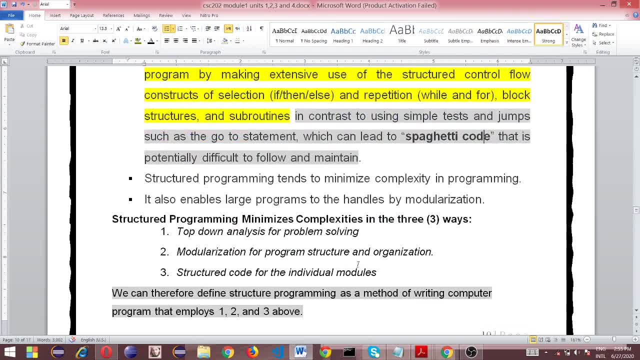 technology new new design for development so now let's see the structured programming minimizes uh structured programming tends to minimize complexity in programming it enables large programs to be handled by modularization 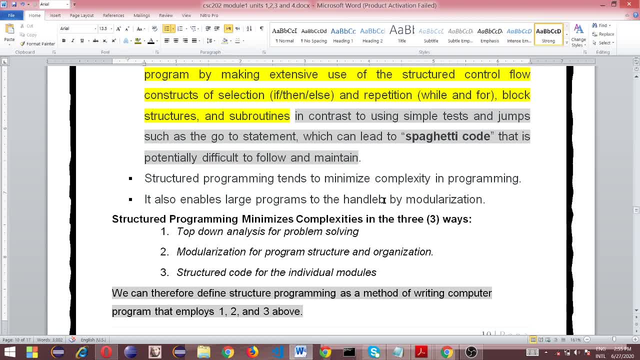 so uh structured programming minimizes complexities in three ways see all we're trying to do is to minimize complexity the program given to you 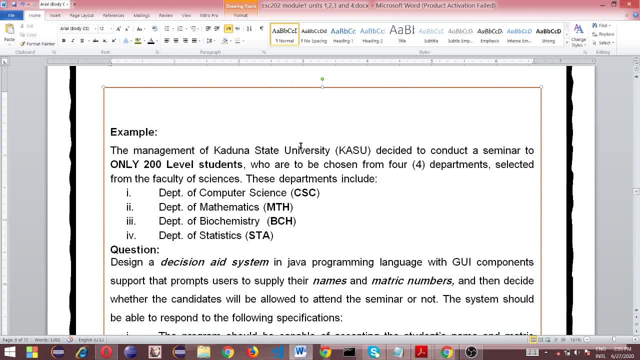 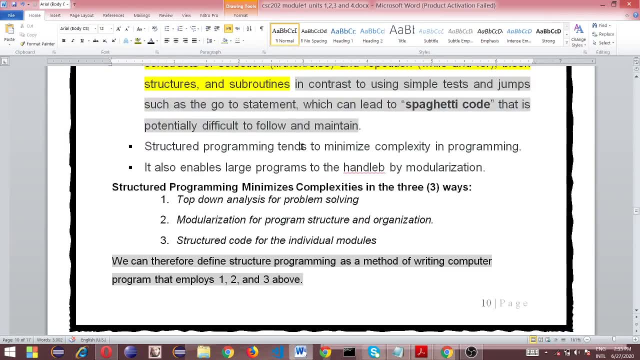 it's very big like this question which is the big one so it becomes complex so there is a need for you to devise ways of minimizing complexity 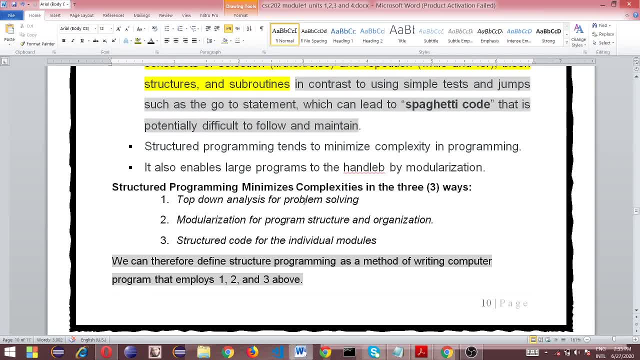 number one is to use the top-down analysis for problem solving or top-down design as we've mentioned that has been explained and then the modularization for program structure and you modulate you put you create models for what the program and then structured code 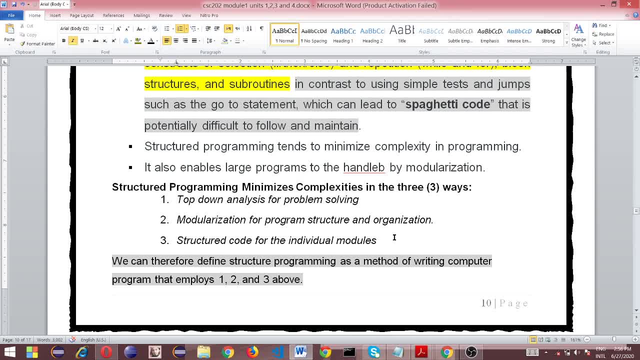 for the individual models each and every module you give it you pick the model and introduce the structured programming uh concept on it the program is complex you do your top-down design 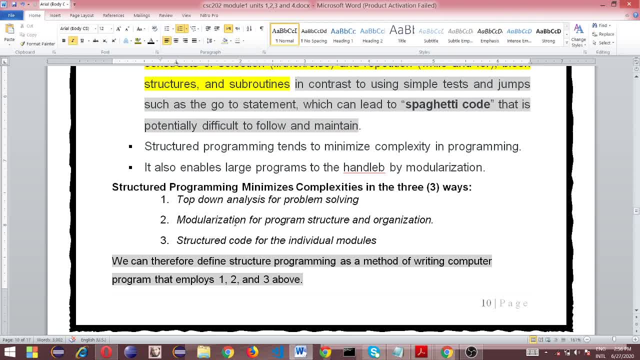 then you pick up your your you create modules for the solution of the problem those modules you created 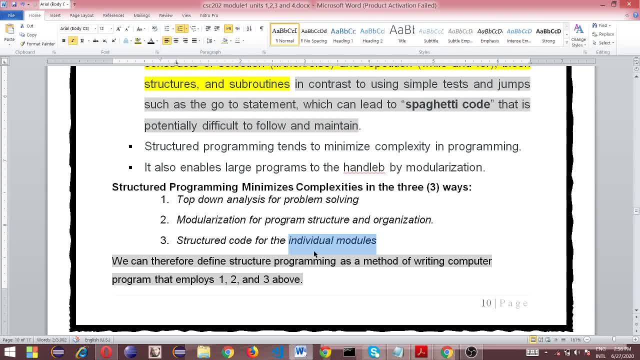 you try to introduce at ev at each and every individual module you try to introduce the structured programming principles structured programming 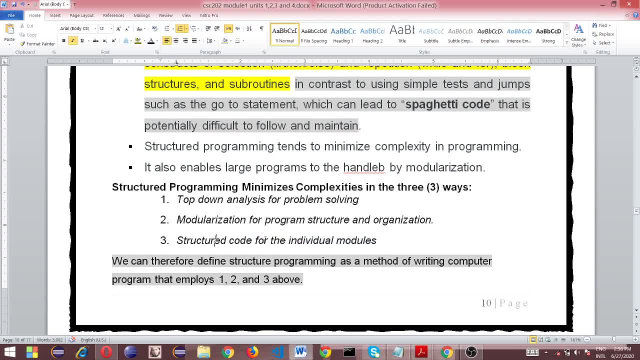 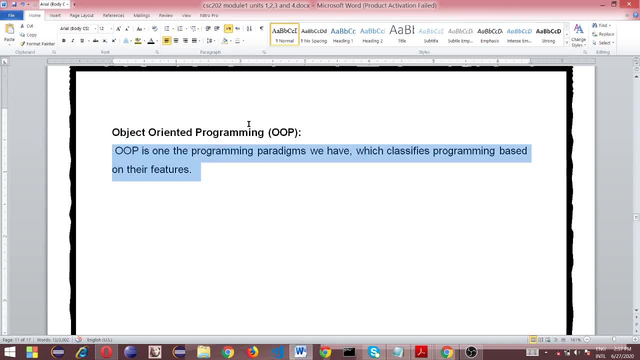 drawings and rules and then that becomes simplified and then also you can also use the object oriented principle or object oriented programming to reduce the volume of 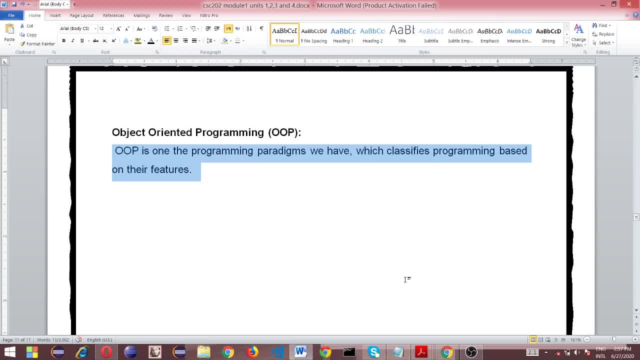 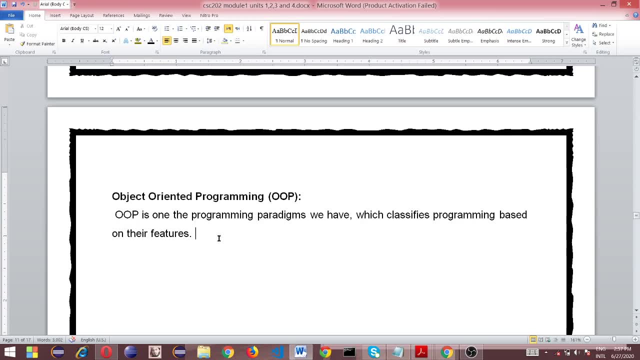 or to reduce the complexity of the program or problem solution you find it you try to find out we shall talk about object oriented programming at the end of this at the end it should be the 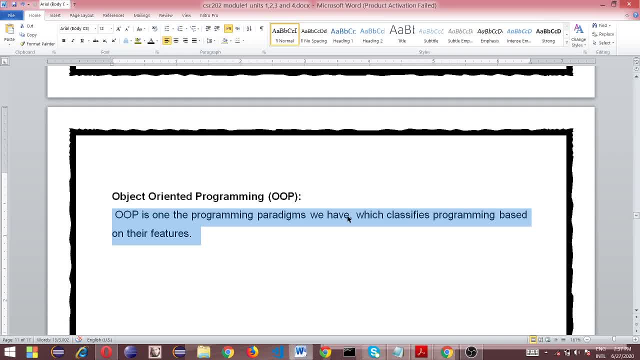 last item we are going to discuss in this course and you also have a pro a program a course called csc 313 where you will learn 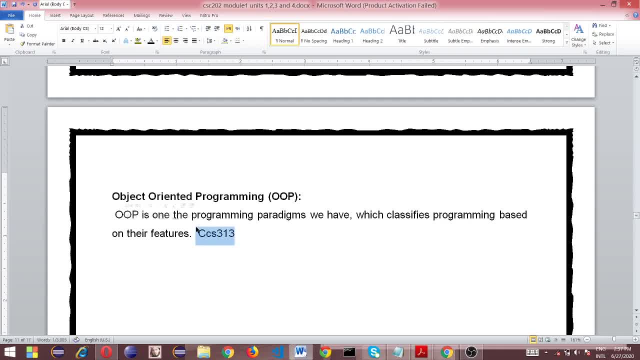 where it is term oop object oriented programming you will learn object oriented programming proper 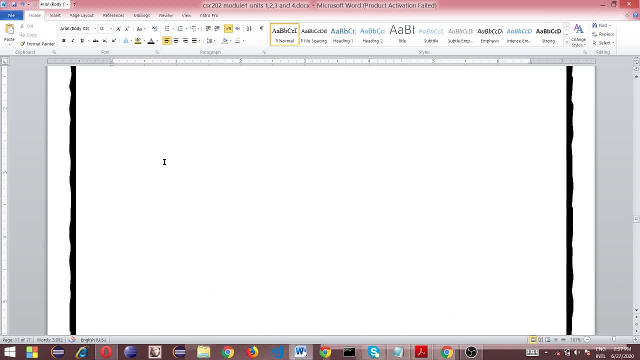 in 300 level so i'm not going to waste time here discuss it but then we'll discuss it along the line 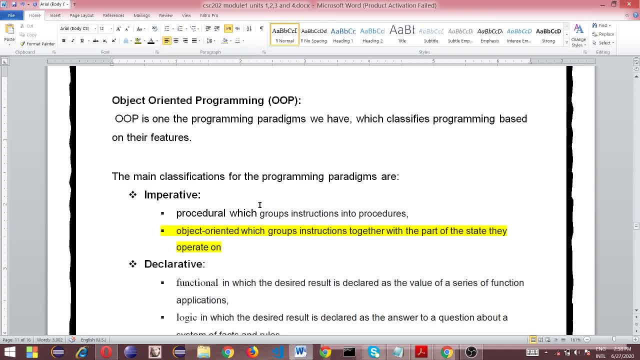 uh so probably you think you know you see we've been talking about these uh object oriented programming structured programming all these functional others all that all that we have mentioned the centered around object oriented programming structured programming functional procedural and whatever is under uh 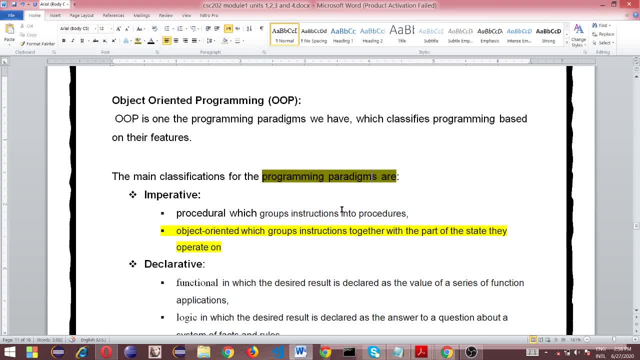 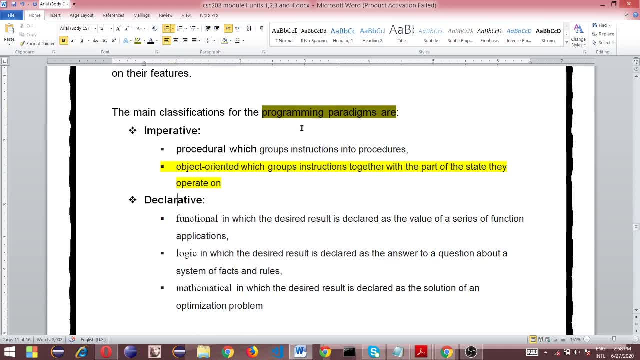 what is being called programming paradigm programming paradigms are many we have the imperative programming paradigms and the declarative programming products so the imperative contains the procedural and object oriented programming 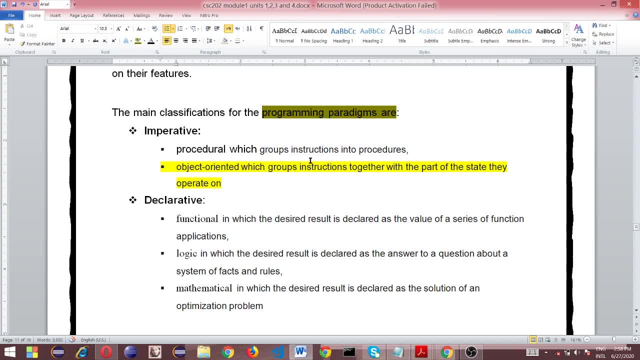 where the procedure it has a group of instructions into it contains group of instructions into a procedure procedure could be this time in the terminology of object project oriented programming means or 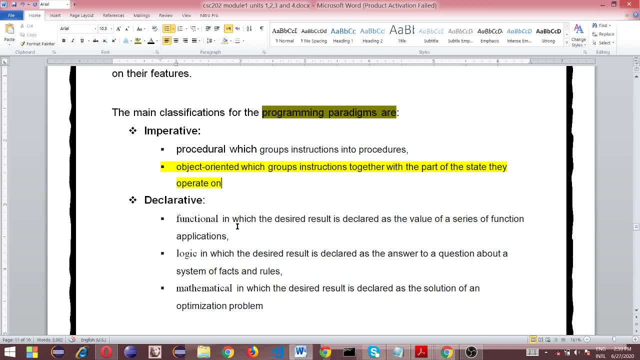 method method does procedural or function if you like so then object oriented programming also is part of imperative this resembles the world the real-world objects where an object has a state and behavior the object function it has a state it has behaviors it has its own properties and it has some functions so and then we have the principles of object oriented 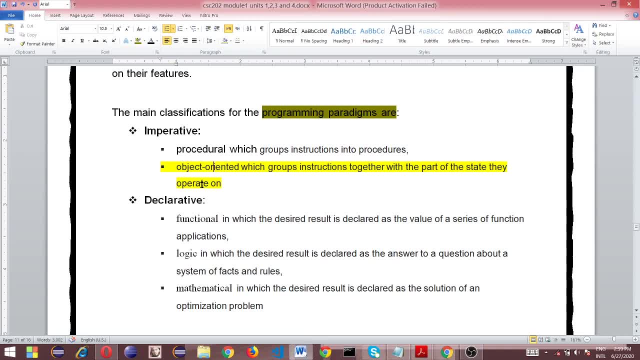 programming and then we also have some 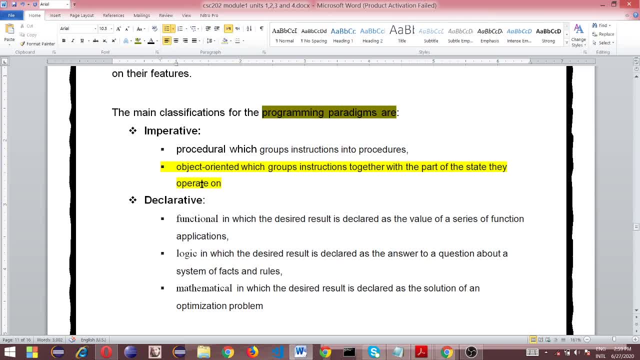 two things that are inclined to the objects as I said like the states the member functions the variable function order actually I'm not going to waste my time 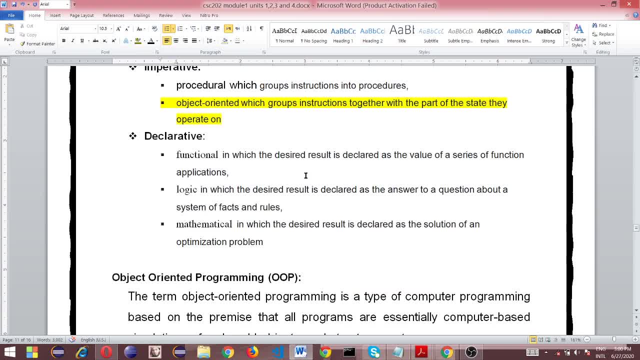 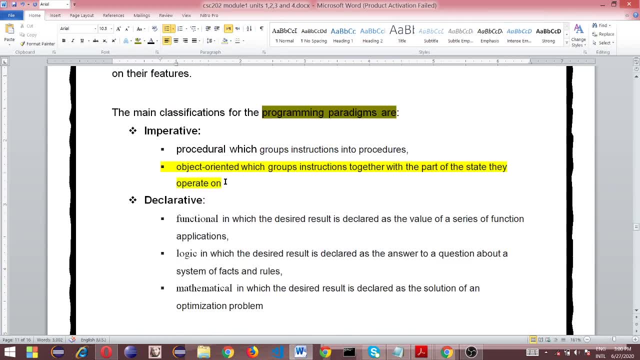 here because it is no yet time I will discuss each time permits and then at 300 level have a very good discussion about it and clarification and then the 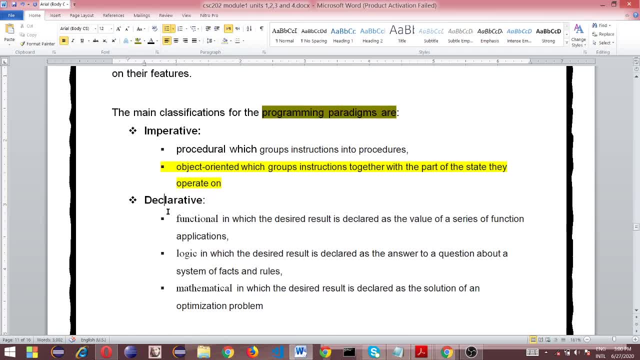 other category of programming paradigm is declarative programming for them where we have the function of object oriented programming and then we have the 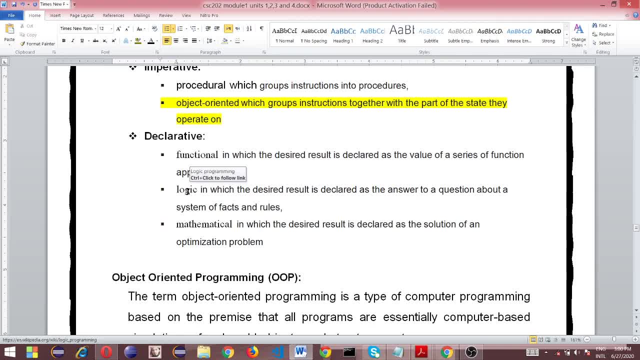 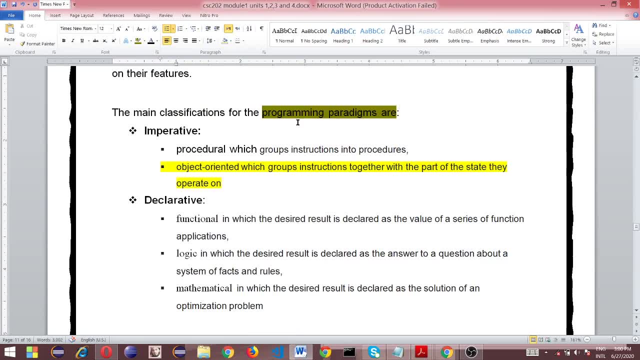 functional programming paradigm and then we have the logic and then we have the mathematical programming program please go to programming paradigms and learn 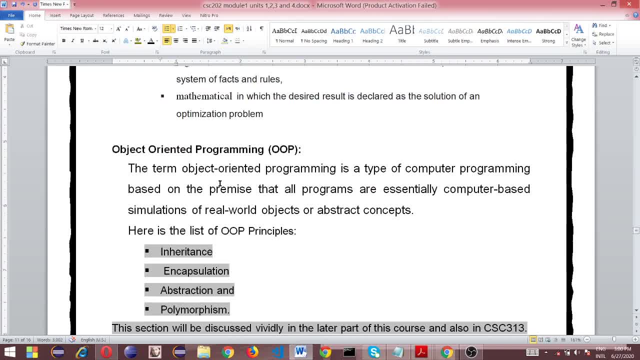 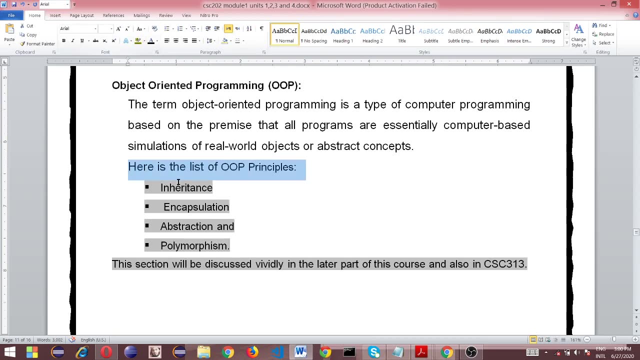 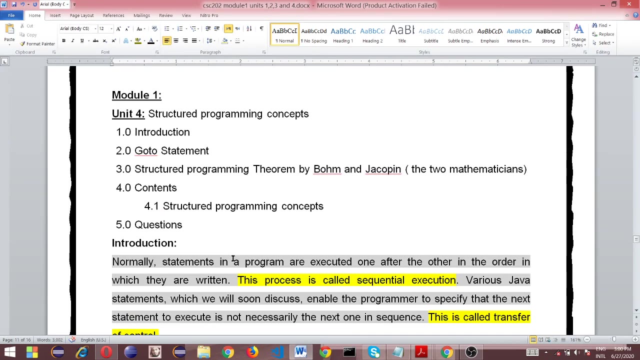 more object oriented programming the term object oriented programming is the type of programming based on the premise that all old programs are essentially computer-based simulation of real-world objects or abstract concept and then the principles are mentioned here it inherits the encapsulation, polymorphism, the abstraction these will be discussed as I mentioned for buying 313 and part of 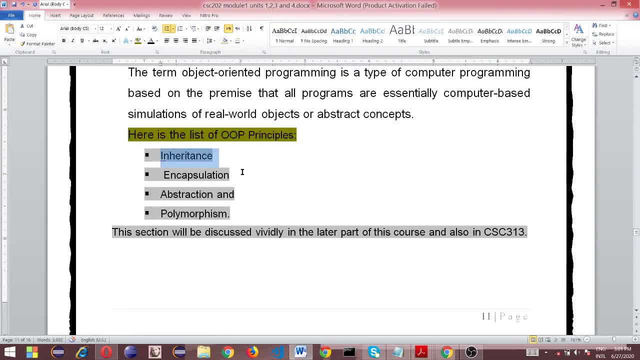 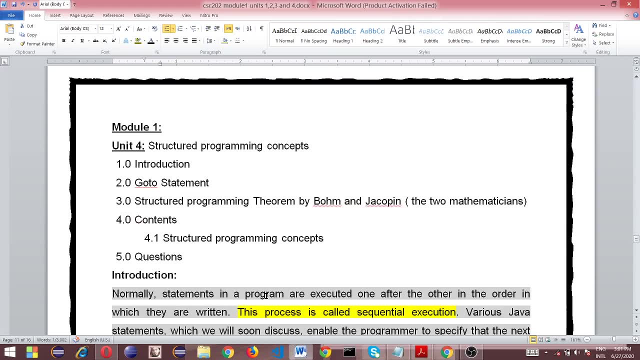 part of them like for example the inheritance and encapsulation would be discussed in this program by the term in 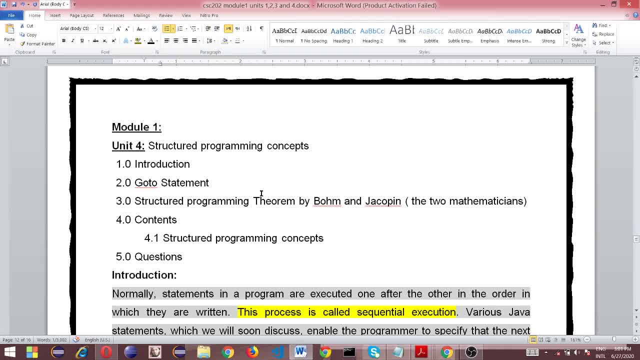 so now structured programming concepts We are now trying to discuss structured programming What is structured programming The introduction the go-to statement the structured programming theory by the Boehm and Giacopini The two mathematicians and then the structured programming itself and some questions for you to practice here 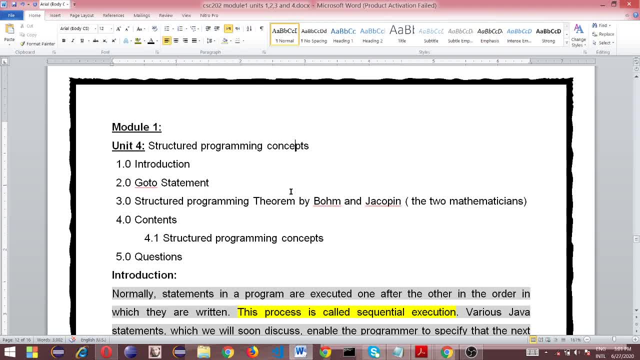 Actually if you talk about structure You 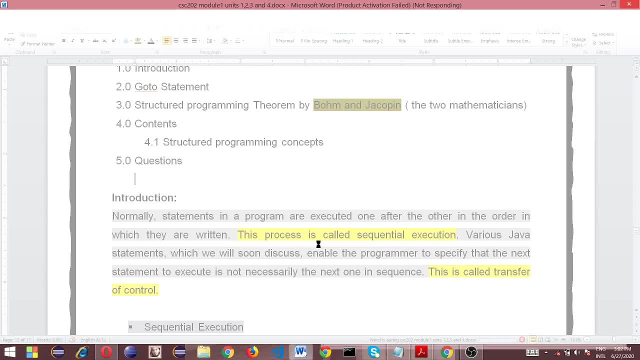 But then there are situations whereby The execution of the program is is not required to be sequential or serial The first one I mentioned is serial, but there are situations whereby it is not meant to be serial rather It is meant to be selective 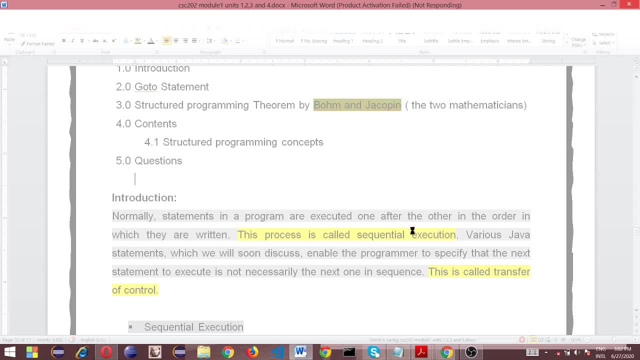 It's the programming needs to be branching It needs to be jumping rather actually use that word it branches from one line number to another line number 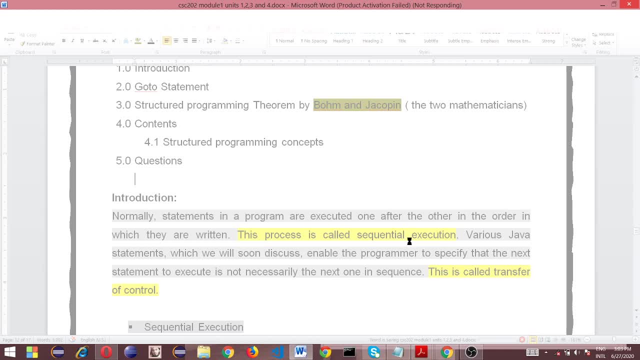 Based on some conditions with the aid of some conditional statements I'm sorry 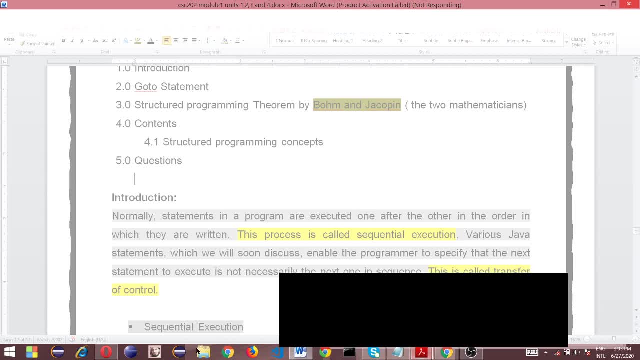 I'm sorry, but this image word got problem. Let me quickly open the other version of PDF so I don't cut my Don't interrupt the video Something is wrong. I'm sorry 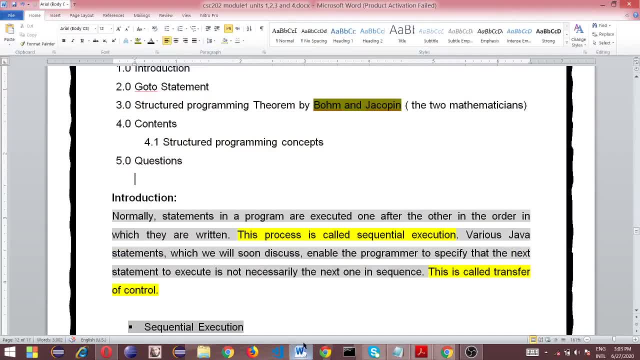 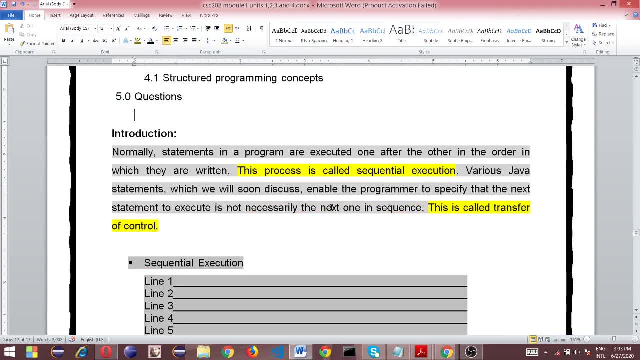 All right, it's okay now, okay, so as mentioned Take in some situation The program need to be sequential if there is no any option no any no diamond sign That is there is no branching. There is no transfer of control It reads from one line number to another line number to the last one But then if Gary's won't call transfer of control so must be 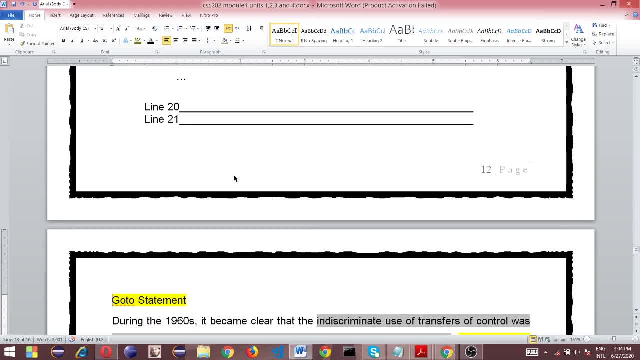 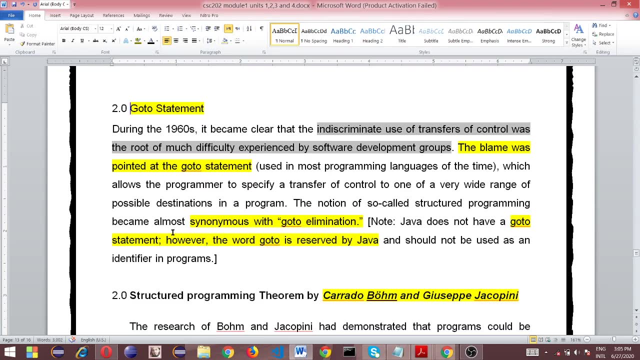 So now let's discuss go to as we mentioned Go to statement here. We're trying to refer to the past What happened during go to statement usage? Okay, but then we don't use it Java I mentioned again here Go to statement in 19 during 1990s it become clear 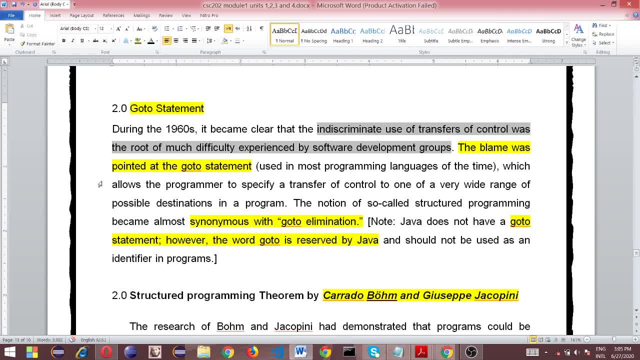 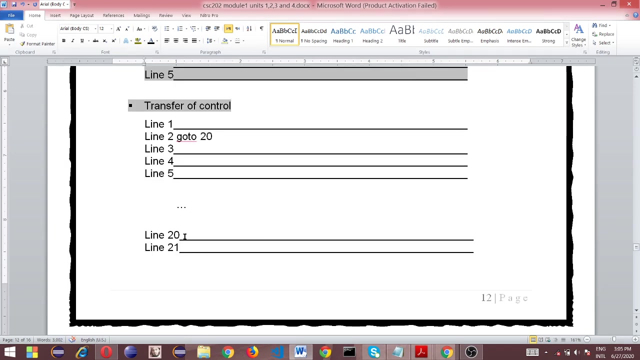 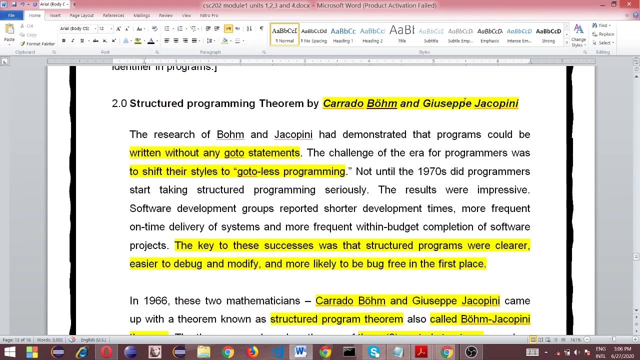 that the indiscriminate use of transfer of control was the was the root of the many or much difficulty experienced by software development group the if you use goto statement if there are goto statement too many goto statement in your program actually going to have some issues so in 1960s it was realized that there are issues and then goto statement was blamed so and then if if we really go to statement is not going to be used then there has to be something in place it has to be replaced by another thing because if actually using structural programming and you can not use goto statement then you must use control structures that is the reality because you need to be you need to be you know branching from one line number to another line number so then the structured programming Turing this theory was developed by these two mathematicians the the carotid Bohm and the Giuseppe Giacoppini is Giacoppini and the Bohm produced or developed a kind of you know children for the 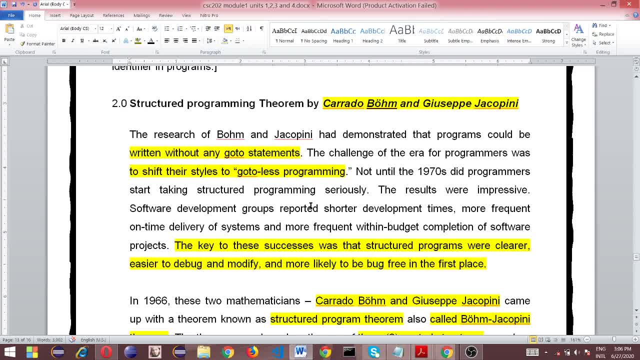 goto statement I mean for these control structures so they demonstrated that programs could be written without any goto statement and they wanted no 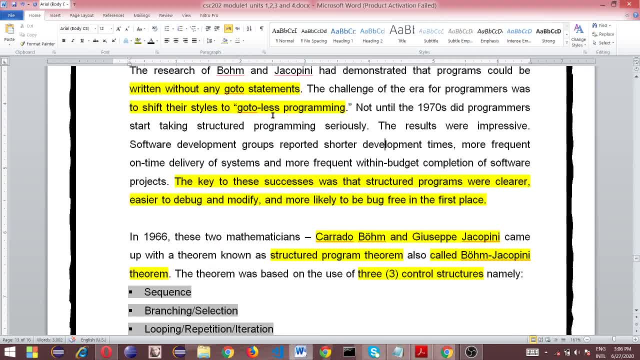 group developers to go to do what they call go to less programming so until until 1970 programmers understood what they mean and they start taking structural programming it took structural programming serious and 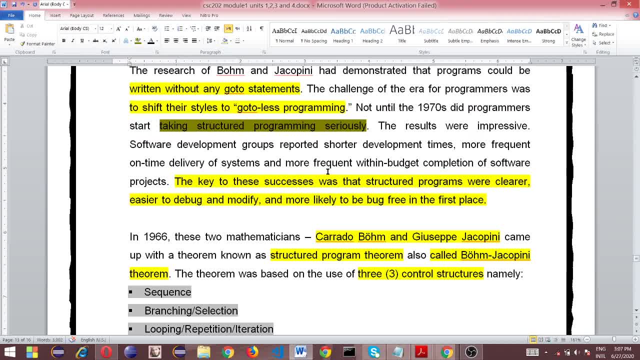 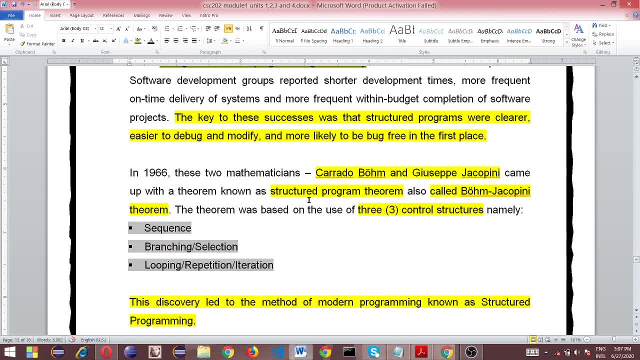 people migrate from such programming style to another programming style the mathematicians came up with a theorem known as structured programming term also called 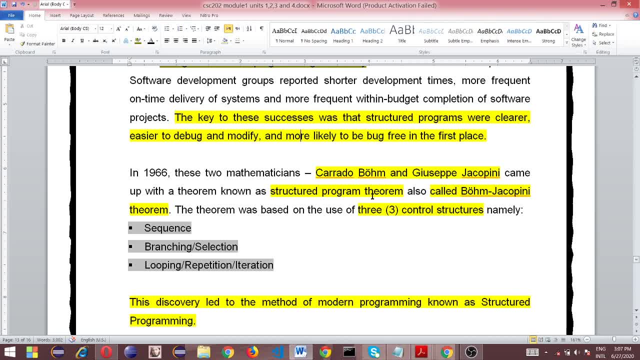 structural programming of course the Giacoppini and the rest these theorems are based on three control structures namely the sequence the branching 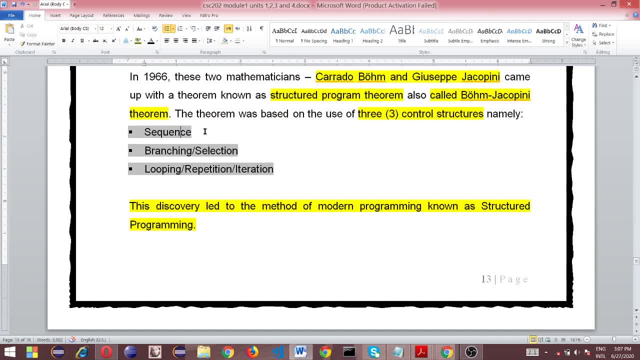 selection and our repetition so we've mentioned that if you are writing program the sequence sequence right or special format of writing program needs the programming to be ready to be executed line by line it is a cute program it is a cute program line by line without any branching 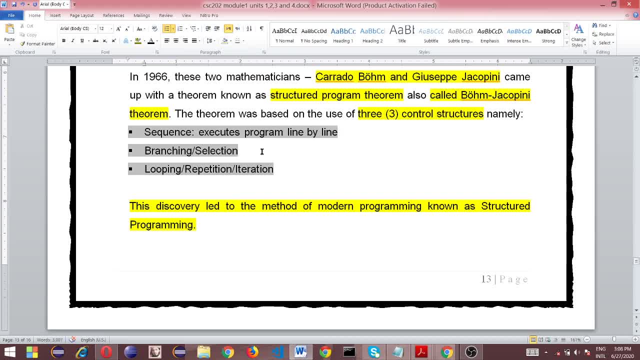 well this one select a particular portion of book you know it's a test it 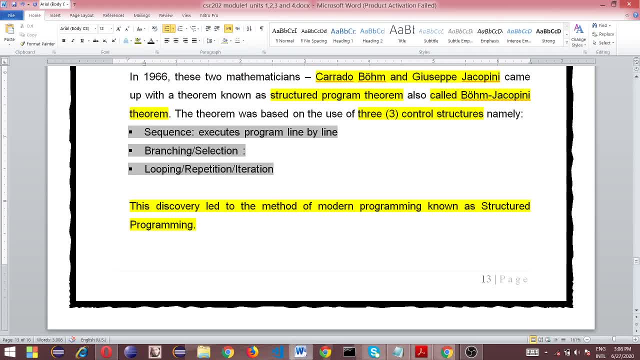 uses it is logical logical statements or logical operators to test for a particular condition if it is if the condition test is true it is accused otherwise it doesn't so you continue to test until 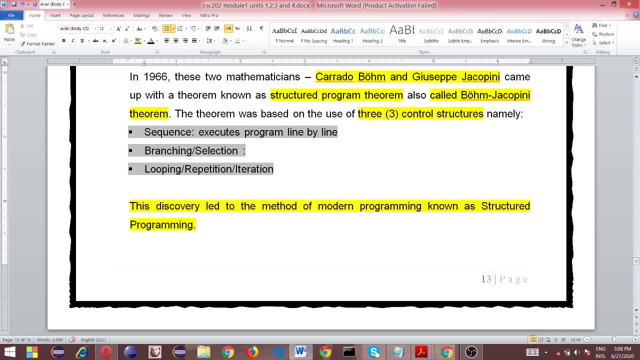 when it reaches to the last so branching test for a condition and looping this tests a condition if it's true 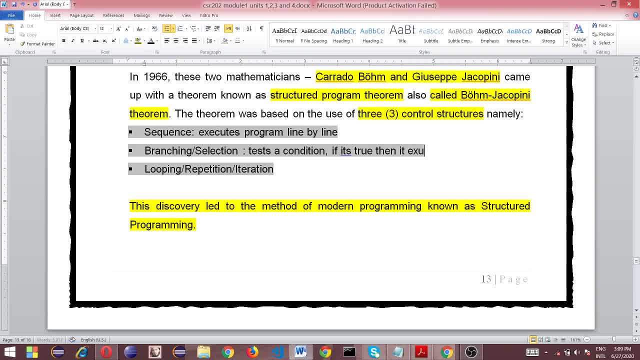 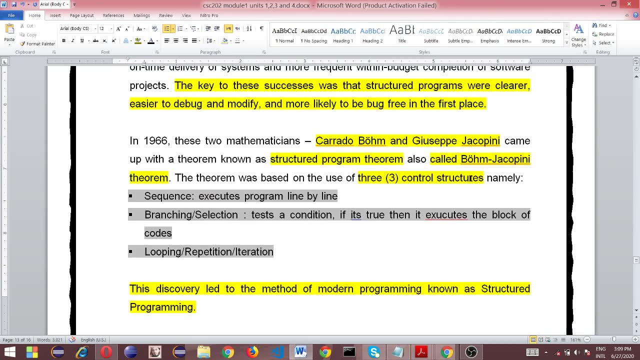 then it executes the block of course otherwise it doesn't or it test it tests for another another condition and 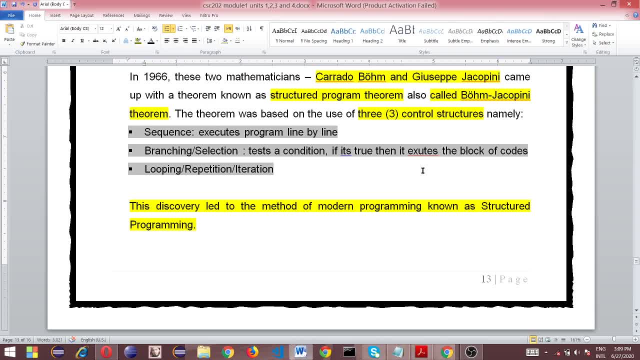 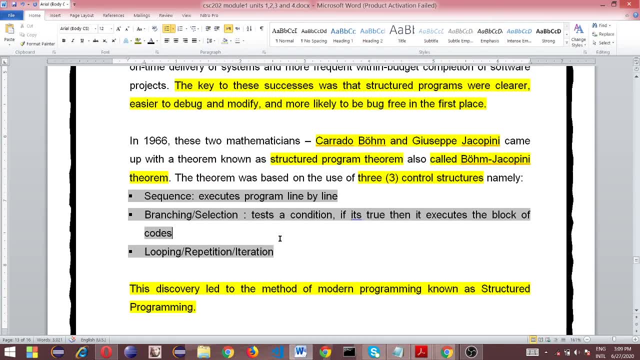 get it as tutor and the iteration of looping keep executing 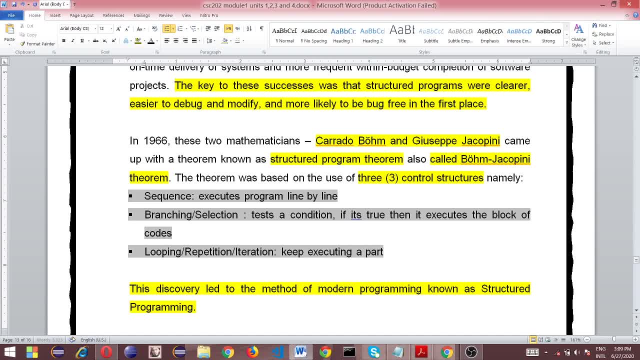 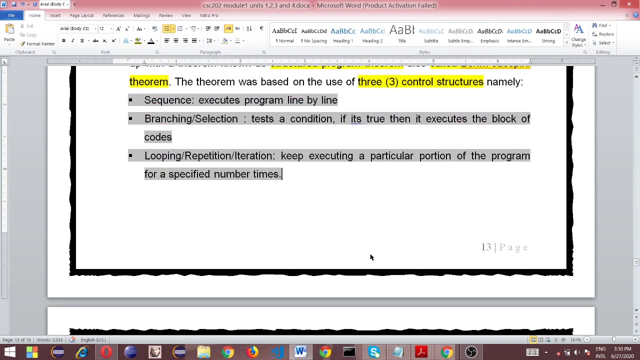 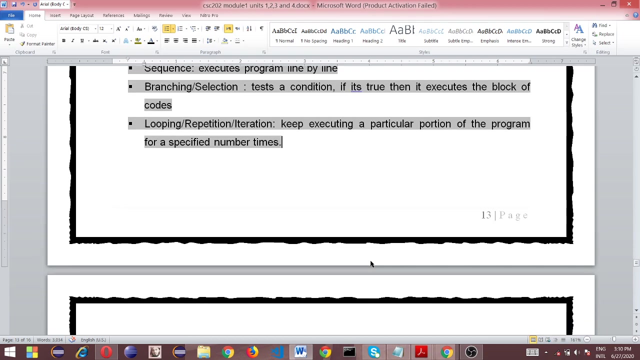 a particular portion a particular portion of the program for a specified number of or a specified number of times even though we have endless loop endless loop is not a good programming practices whenever you are setting up a loop you try to logically cut it or break it so this